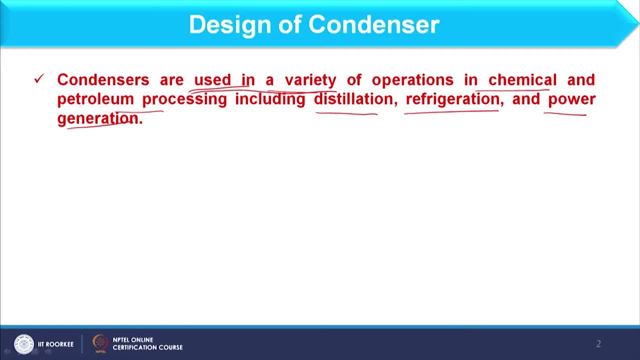 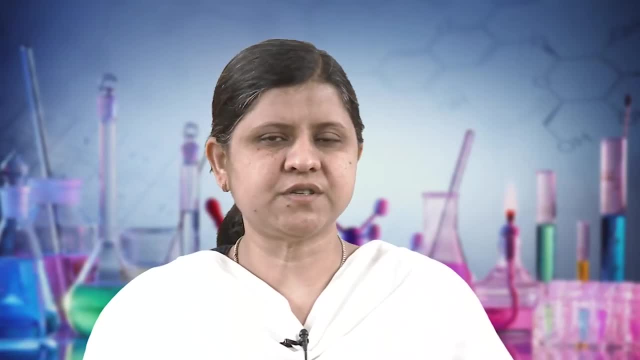 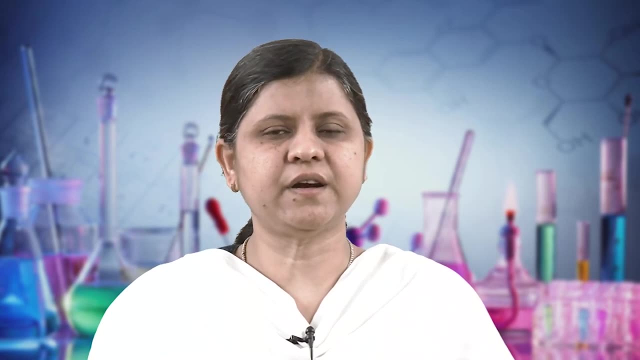 in different industries or different processes, as we have already discussed, right? So as far as distillation is concerned, virtually every distillation column employs either a partial or total condenser. okay, and in that way it converts vapour into liquid. okay, And 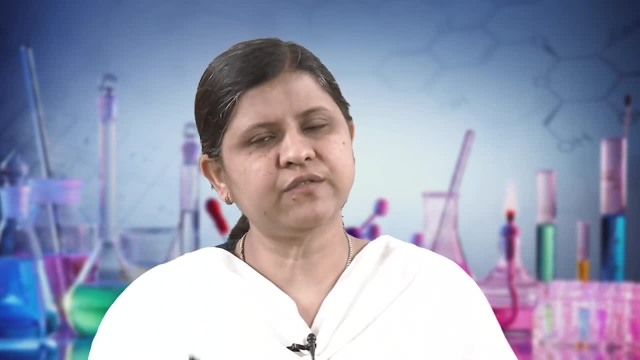 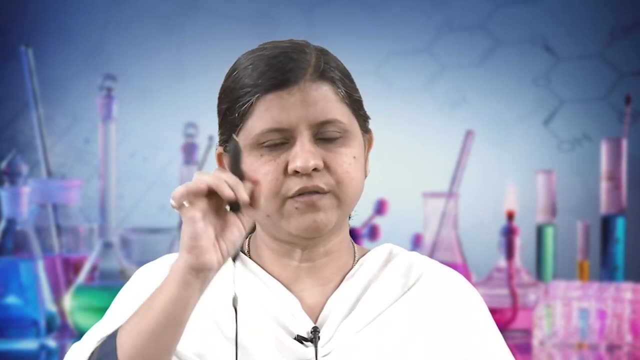 if you understand the process of distillation, we can say that distillation is a process in which the placement of condenser in distillation column. it is basically placed at the top of the distillation column where whatever vapour is generated in distillation column it is. 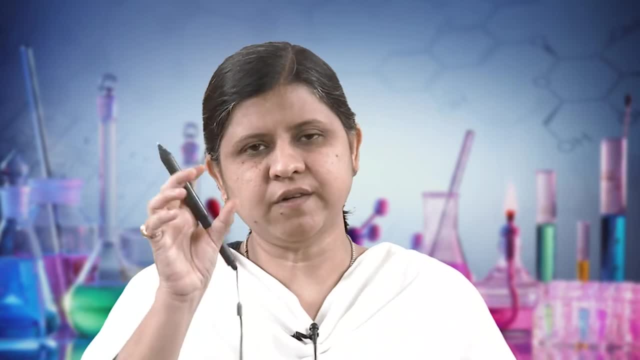 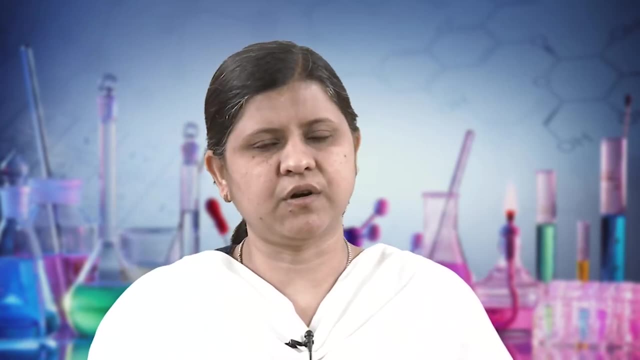 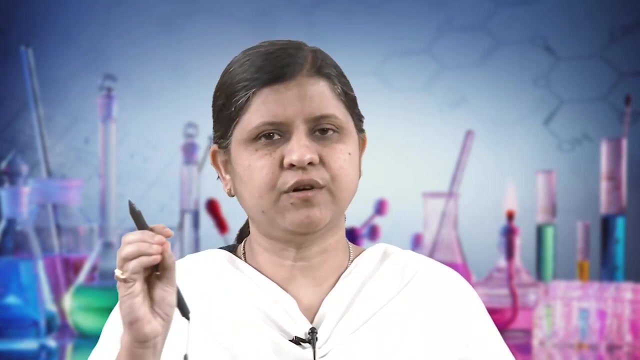 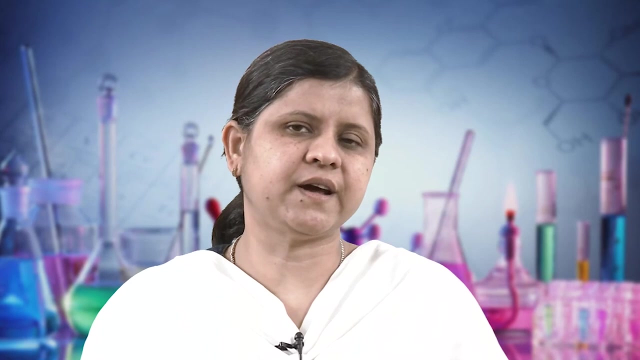 converted into liquid. okay, And what will happen after that? some section of that liquid recycles back to the distillation column and which we call as a reflux right, And at the same time, some section of the condenser we can call it as a top product. okay, Now if I ask you that, what is a total condenser? 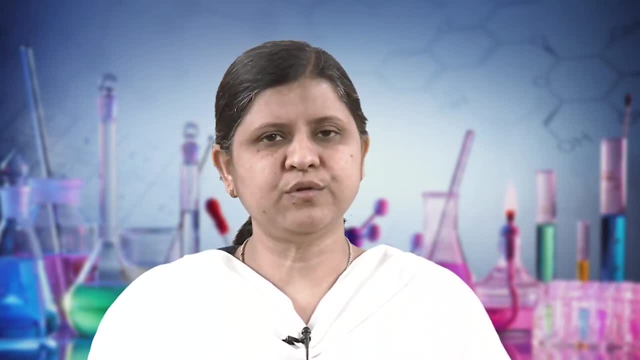 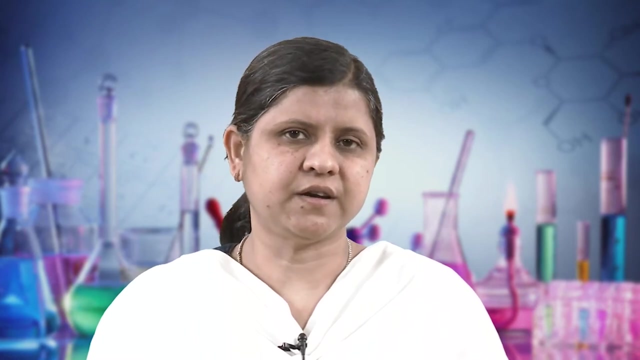 and what is a partial condenser? okay, I hope you know that, but let me further explain it to you, okay? So, as far as partial and total condenser is concerned, it entirely depends on what phase of product you want, right. What phase of product you want right, What phase of product. 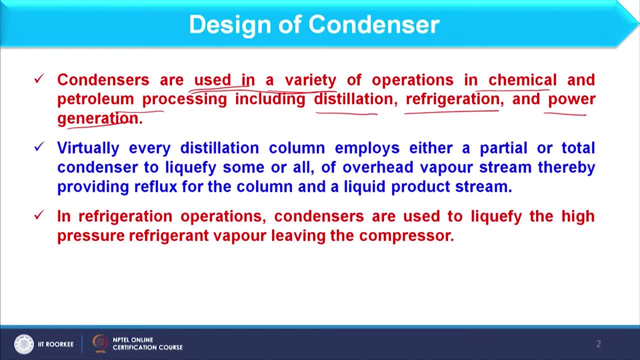 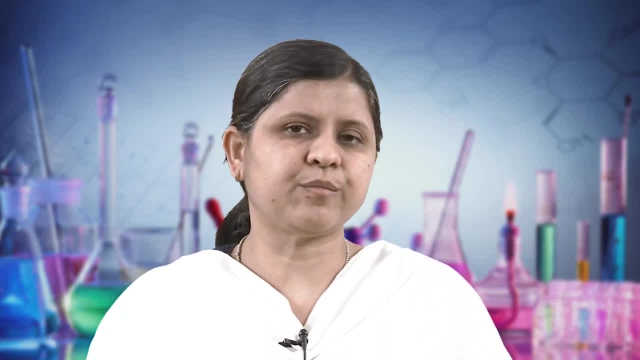 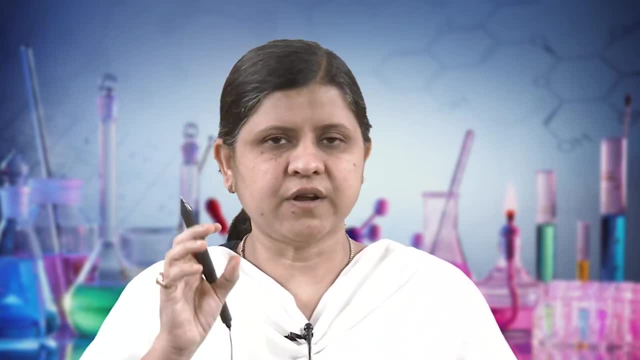 you want from distillation column as top product, okay. So what will happen when I say that you can? when I say that your product should be in vapor form? okay, So what you can consider that whatever vapour you can take as a. so what you can do over here, you 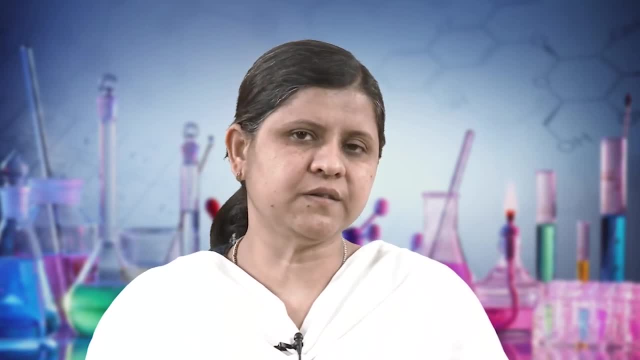 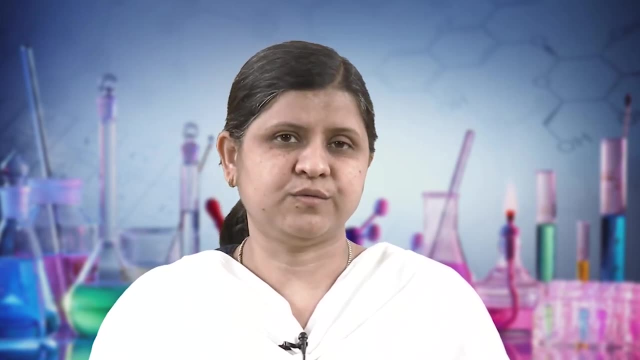 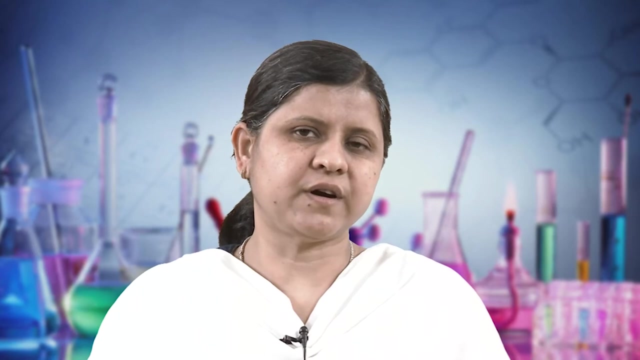 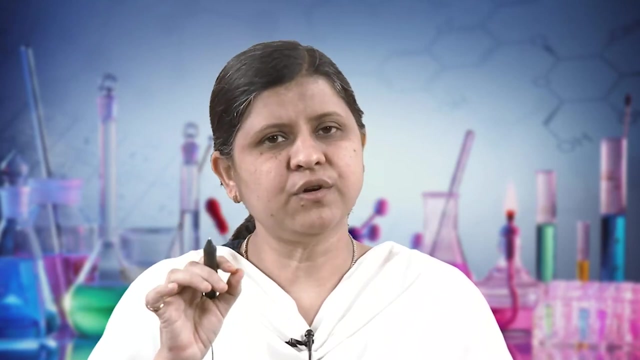 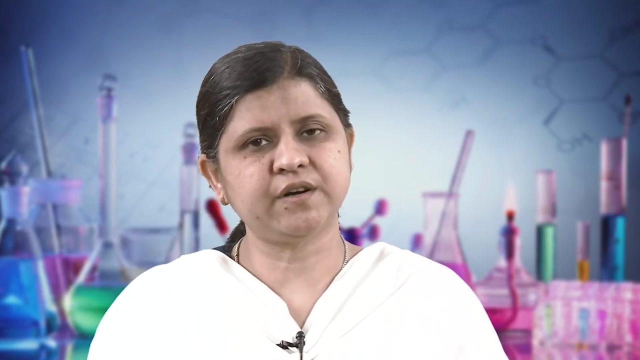 can consider whatever vapour is exiting the distillation column, that you can consider as a product, right, but no, because what will happen if I ask you that you should consider product in vapor form? okay, But then also you require some liquid, because that liquid should return to the distillation. 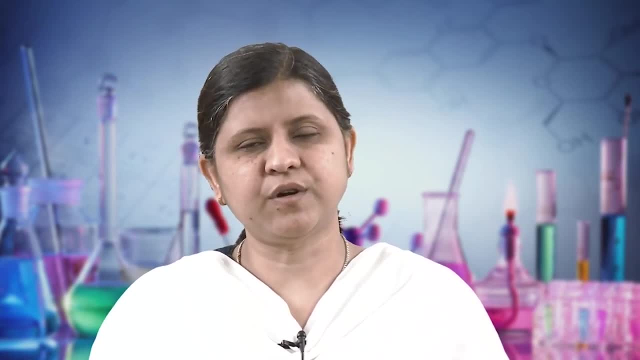 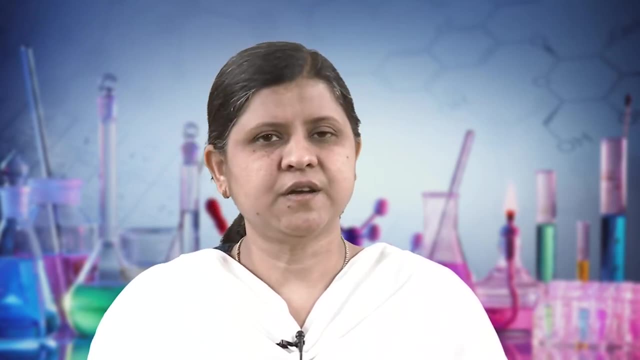 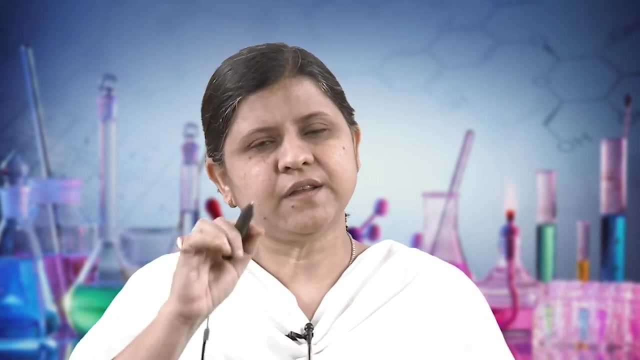 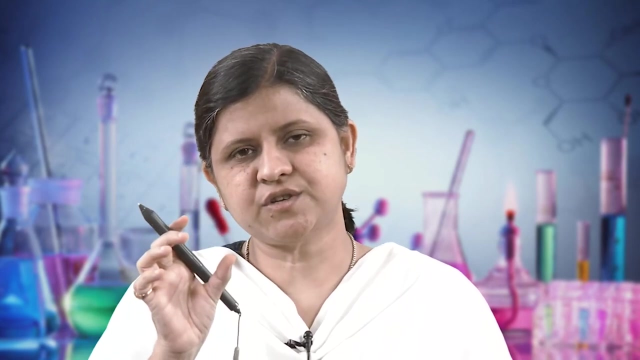 column as a reflux, because until, unless I am not having vapor and liquid phases in distillation column, the process cannot be carried out right. So if I ask you that your top product should be a vapor, okay, then only the vapor which is exiting from the distillation column. it should enter into the condenser and some section. 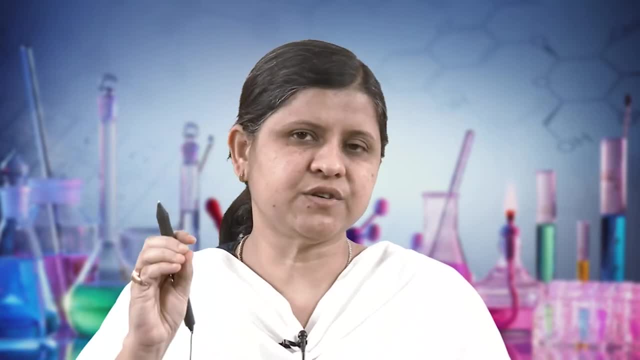 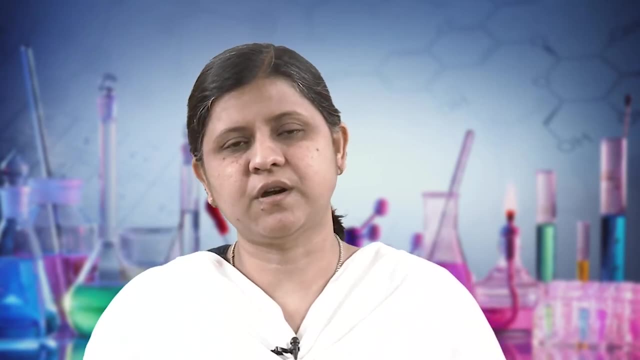 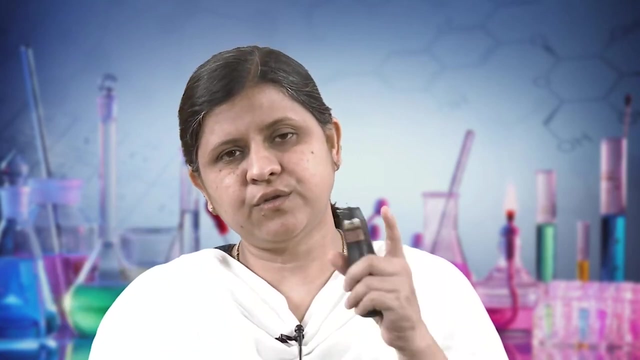 of that vapor should be converted. It should be converted into liquid and that liquid should return back to the distillation column as reflux right and in that case, vapor you can obtain as product. So what you have done, you have obtained your product in vapor form but at the same time 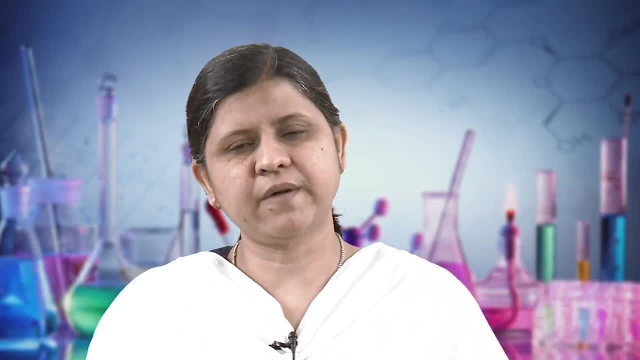 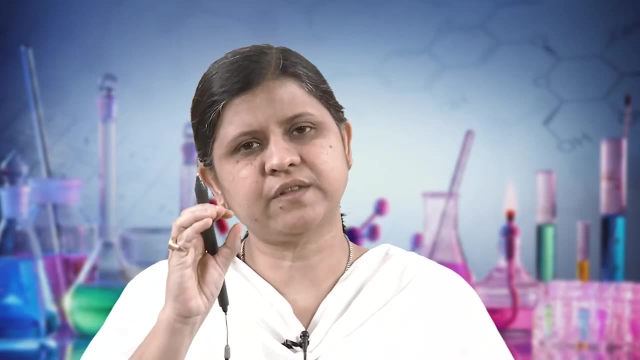 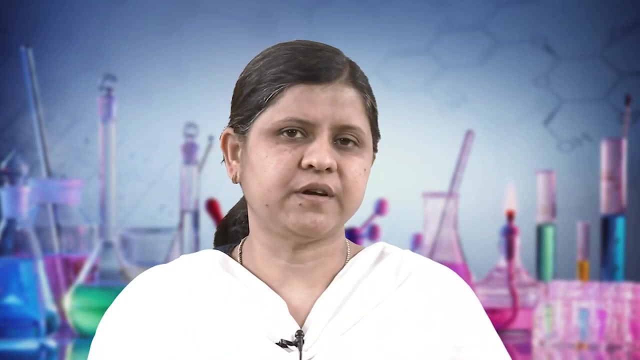 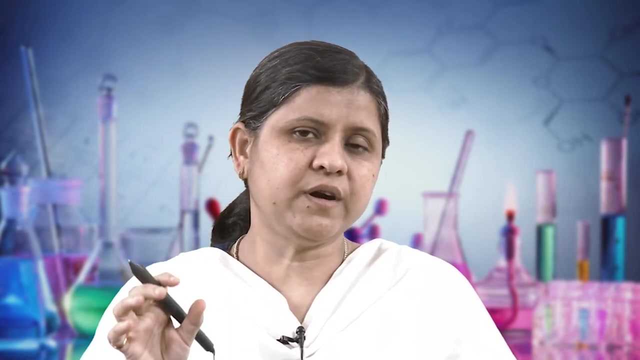 you have returned the liquid to distillation column as reflux. So whatever feed is entering into the condenser, only some section of that vapor is converted into liquid, and that will depend on how much reflux you want, right? So in that case, some of the section of vapor is converted into the liquid and therefore 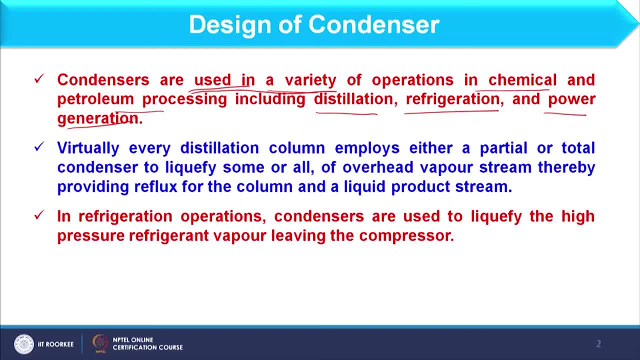 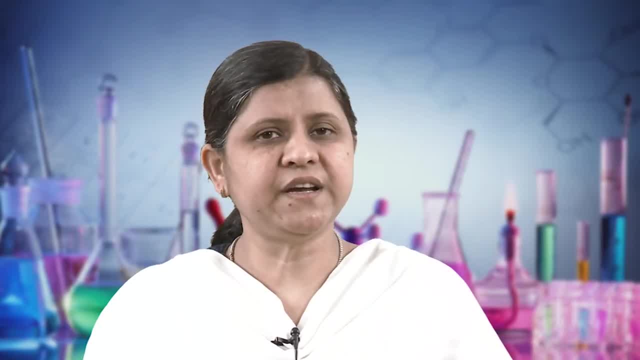 you call that as partial condenser right Now. if I ask you what should be the total condenser? total condenser basically condenses complete vapor which is entering into this, And in that case reflux as well as top product should be converted into liquid. 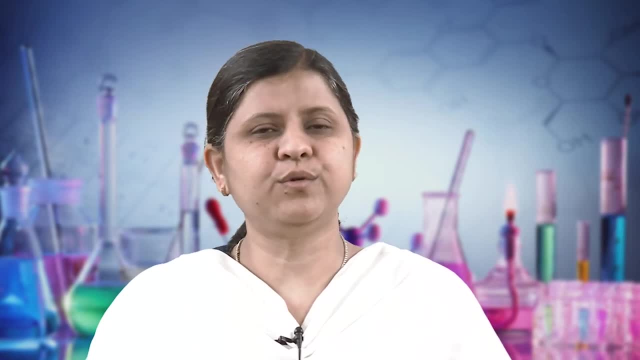 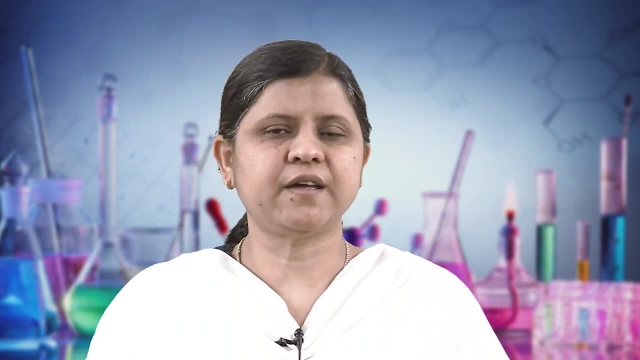 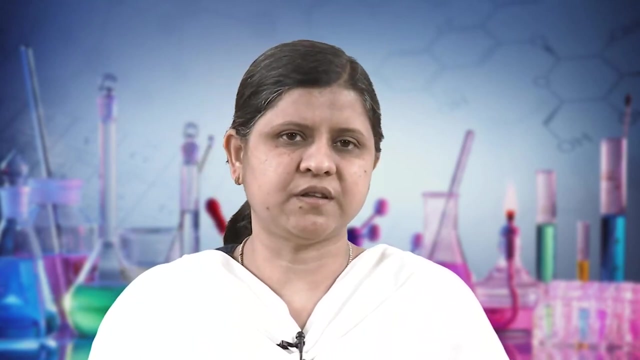 Okay, So top product of the distillation column, both should be at liquid phase. So in that case we consider that as total condenser and if product I want as vapor we consider partial condenser. So I hope you understand the difference between the two. 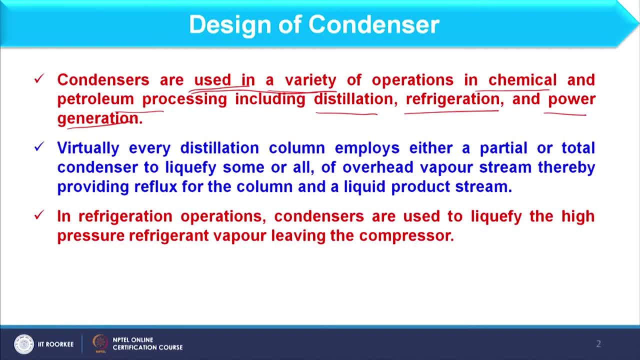 And, as we have already discussed that, condenser use in refrigeration operation is very important, okay, So, in refrigeration operation, condenser are reflux. Okay, So condenser are used to liquefy the high pressure refrigerant vapor, leaving the compressor. 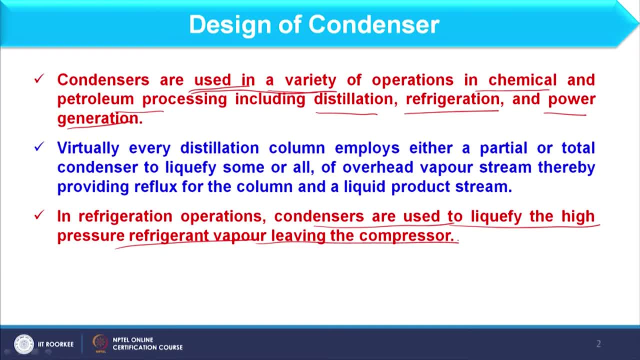 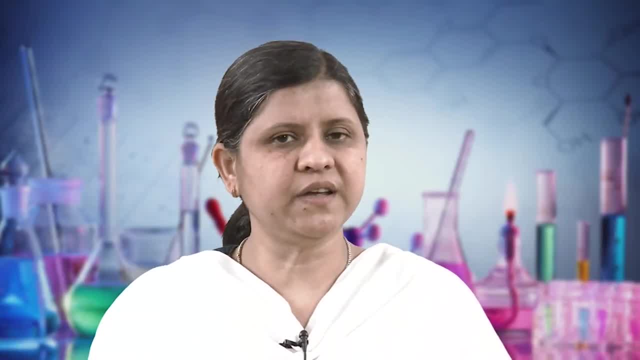 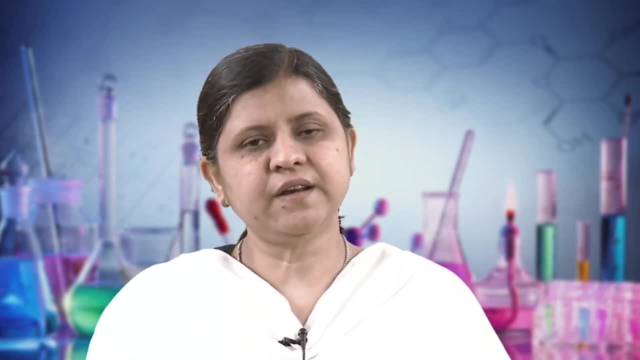 okay. So if you recall the refrigeration cycle, what will happen? Initially we have evaporator- okay, In that evaporator, whatever liquid and vapor mixture is entering from throttle valve- okay, that liquid is converted into the vapor and complete vapor further enters into the compressor. 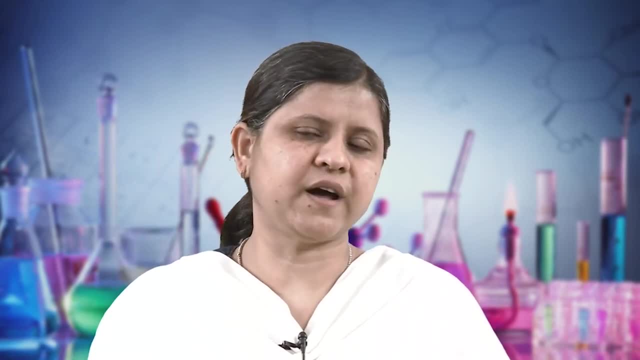 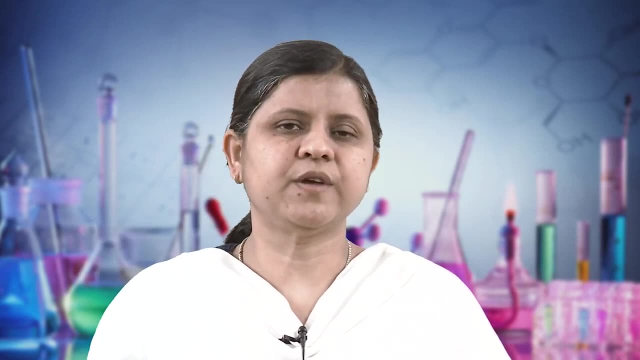 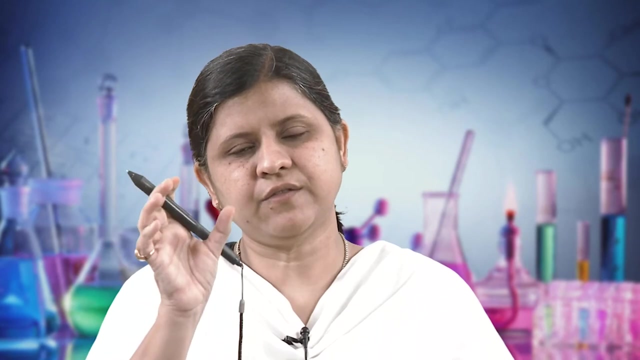 Okay, So the vapor is converted into the compressor, where it is reaching to high pressure and high temperature, and then it is further entering into the condenser, where the vapor gives its heat to the atmosphere. okay, And then after that we have vapor, and then after that vapor is converted into the liquid. 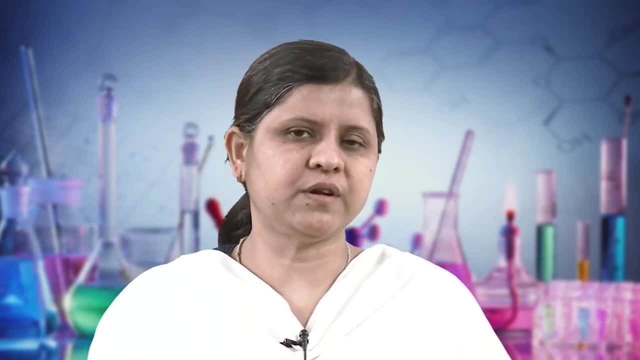 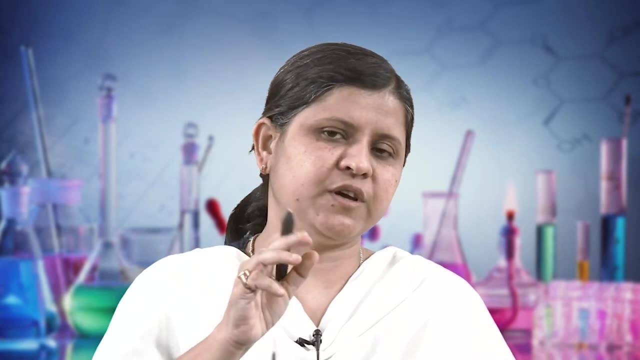 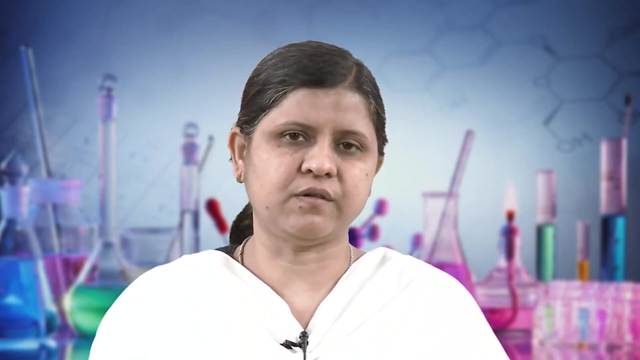 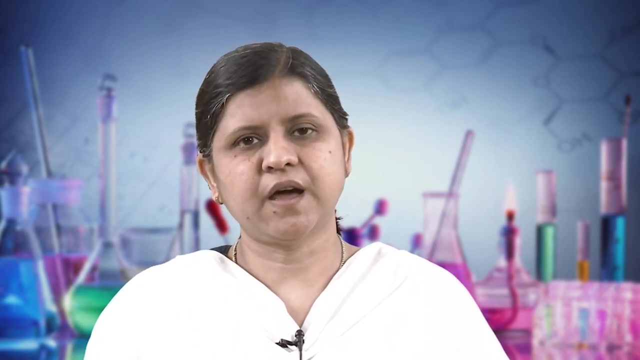 and that liquid is further entered into the throttle valve, where sudden expansion gives vapor as well as liquid, and that vapor-liquid mixture is again into the evaporator. So you see, we have evaporator, compressor, condenser and throttle valve. okay, This is basically the refrigeration cycle and, based on that, refrigerators which we are. 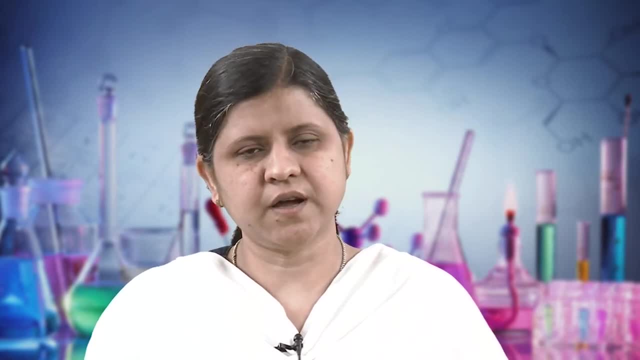 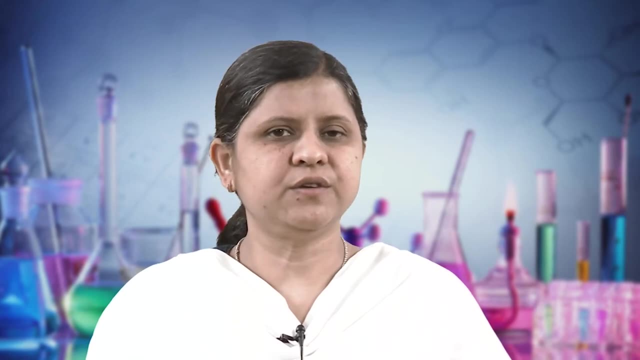 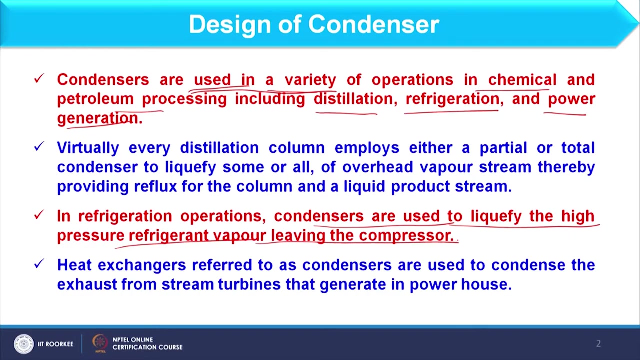 used in our houses. it also works right. So here we use the condenser extensively, okay, And after that we have the condenser, Okay. Okay, We can use the condenser in power generation. okay, Now what will happen in power generation? or let me ask you what will happen in Rankine? 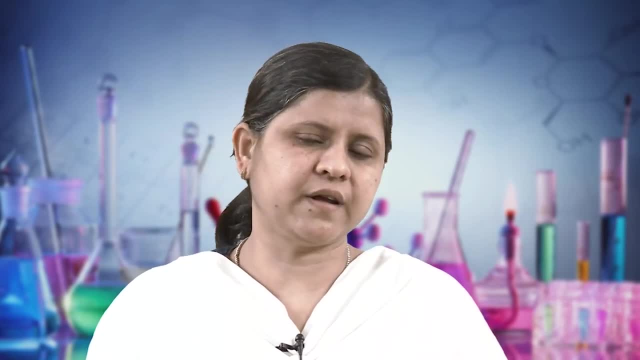 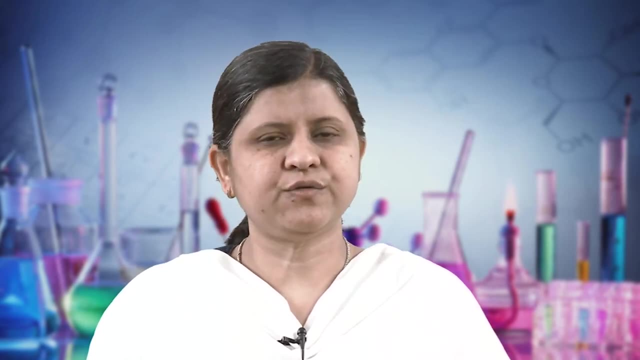 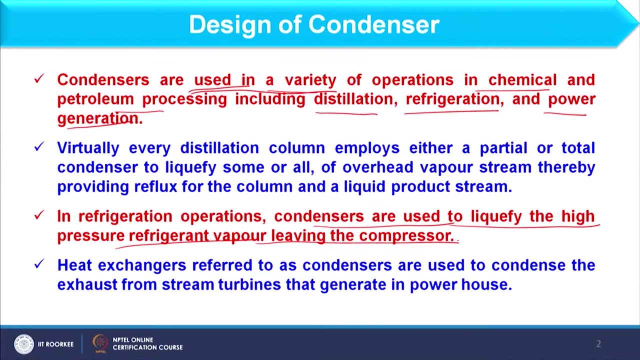 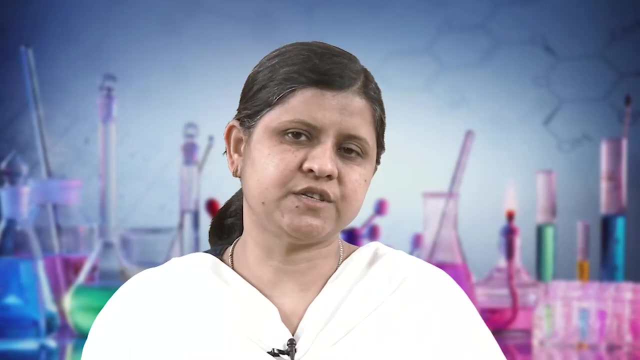 cycle, because thermal power plant works on Rankine cycle principle, right? So first of all, water is basically preheated and then converted into saturated steam in boiler, And after that it is converted into supersaturated condition, and after that it is converted. 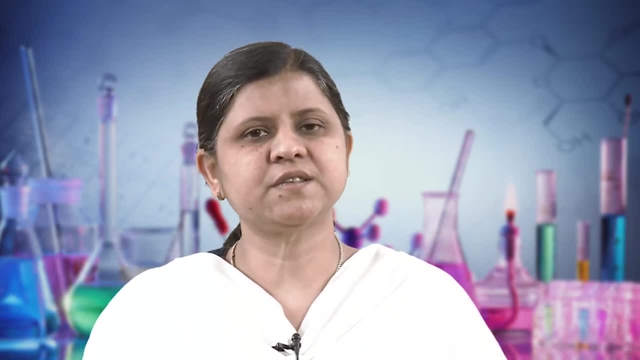 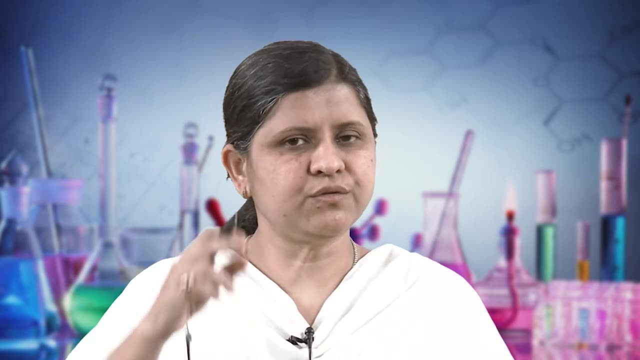 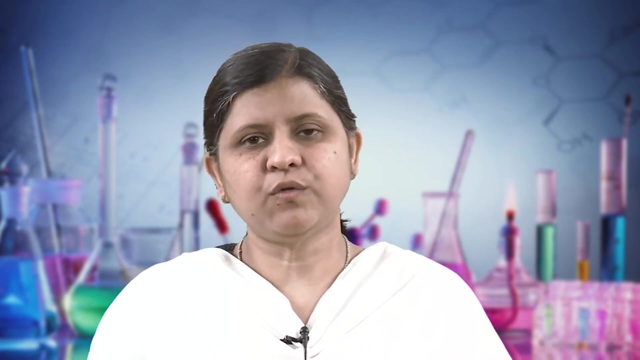 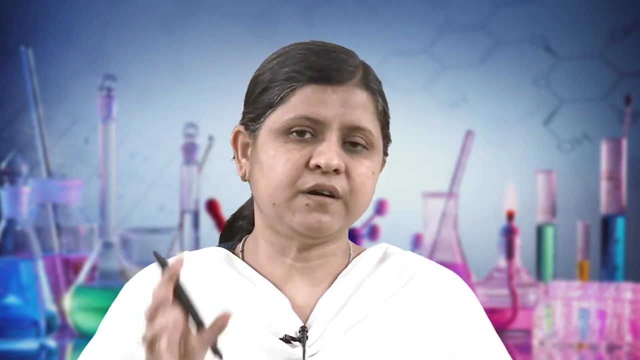 into supersaturated form. and then it is entered into steam turbine where expansion of vapor takes place. Due to that expansion in steam turbine, shaft moves and we can have electricity- right. But what will happen with that steam? Steam is condensed When it comes across the turbine- right, but complete steam is not condensed. 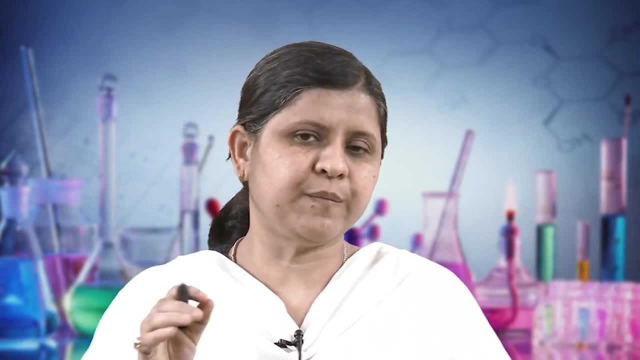 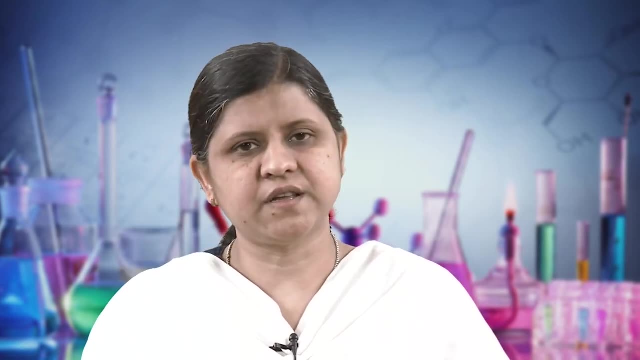 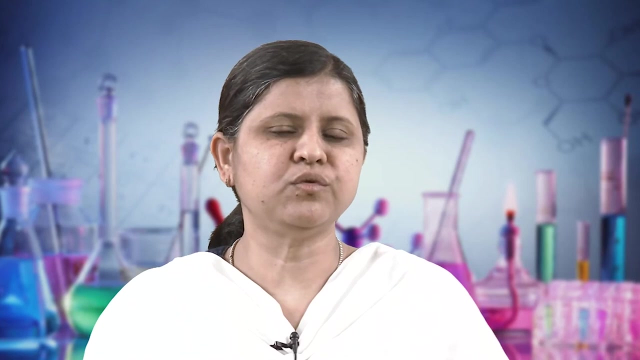 Some vapor will remain there, okay. So what will happen After that? that vapor-liquid mixture enters into the condenser, okay, And whatever vapor is available there that is further converted into liquid, and after that, whatever liquid is generated- Okay. 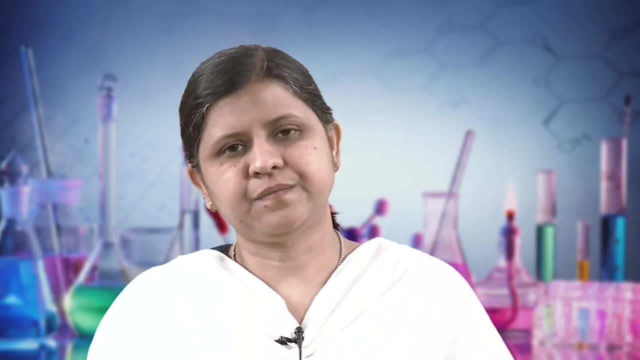 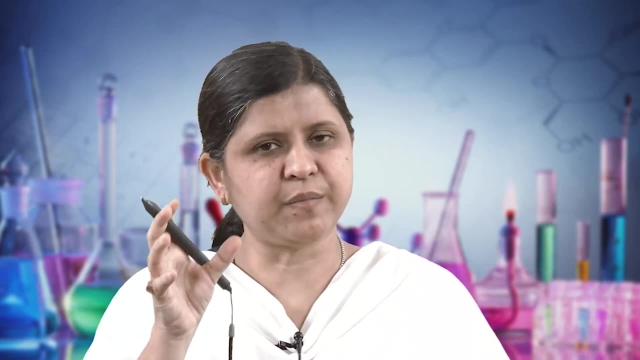 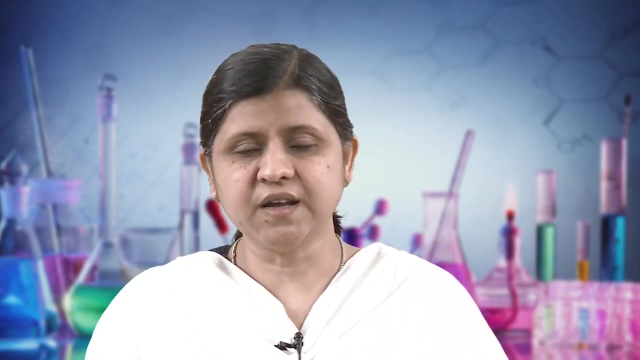 It is further entering into the boiler. okay, So what will happen over here Here, whatever vapor is available in partial form- because some vapor is there, some liquid is there that is converted into complete liquid, okay, in condenser. Now can I directly send this to reboil? 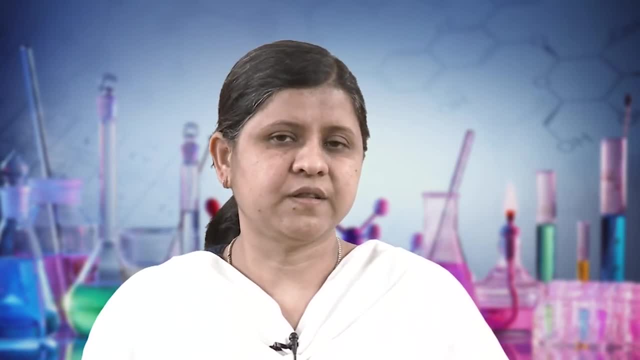 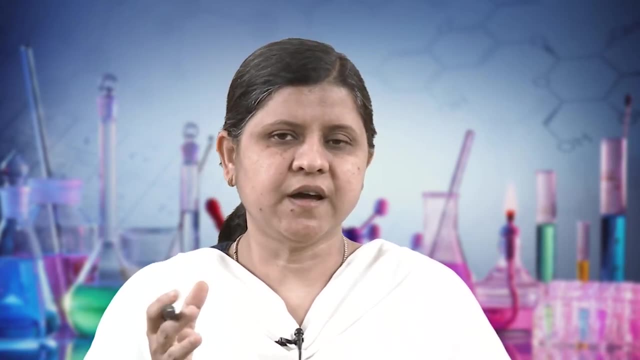 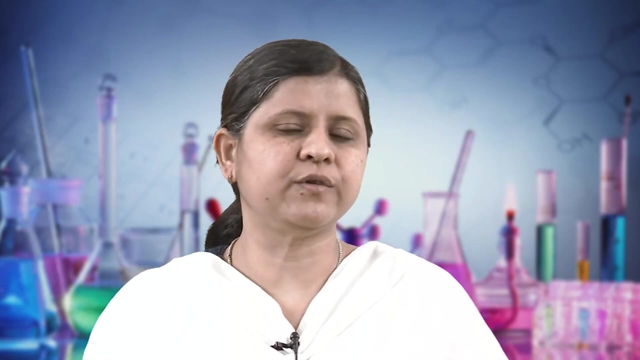 Now, can I directly send this to boiler? The answer is no, Because what will happen? We have vapor and liquid mixture right and when we pump it, okay, it will damage the pump or pump will not work. okay when vapor will be there. 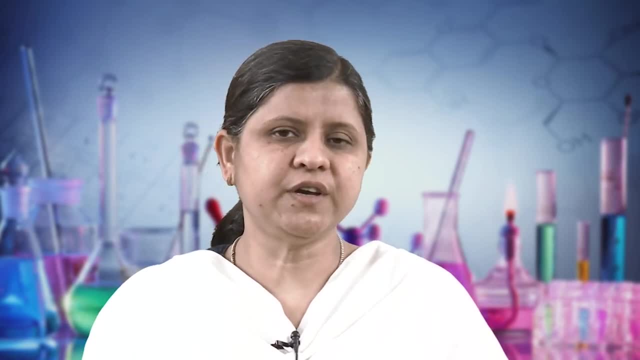 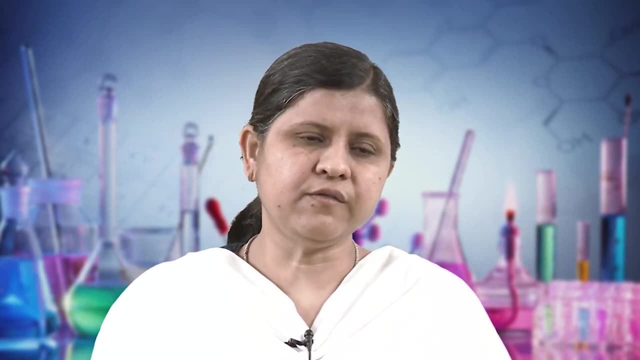 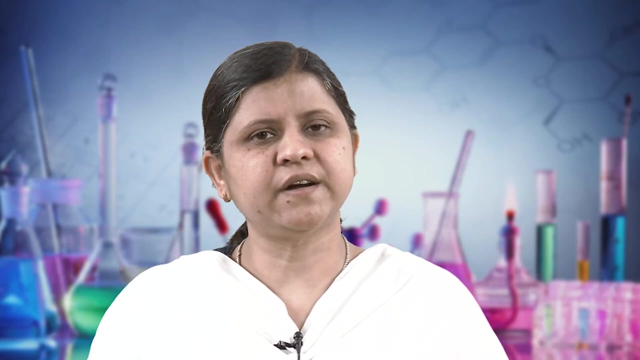 So in that case we have to ensure that feed to the pump is complete liquid and to ensure that we use condenser, where all vapor is converted into the liquid and then it pumps to the boiler right. So in this way we can use condenser in distillation column, in refrigeration cycle and Rankine. 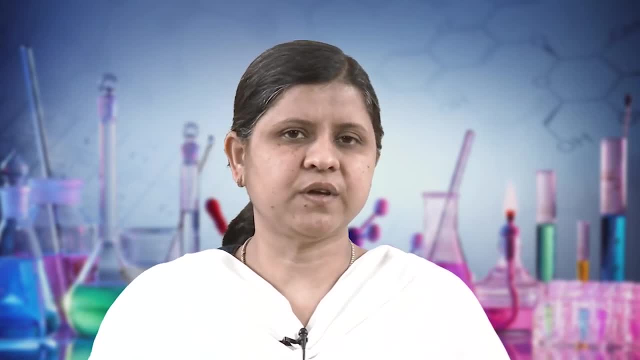 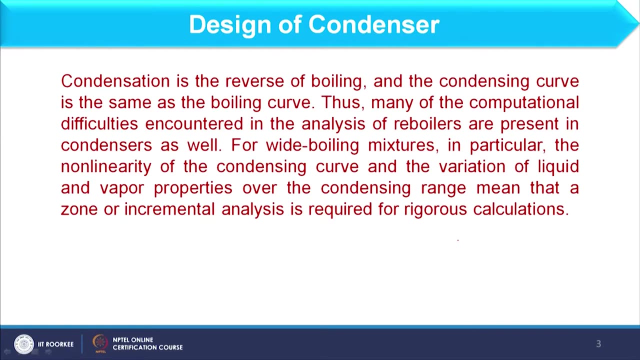 cycle, that is, the power generation cycle. okay, So these are some of the uses of condenser. Now let us further discuss few facts about condenser. okay, So you see, condensation is a reverse of boiling. okay, Boiling we generate vapor and in condenser we generate liquid. 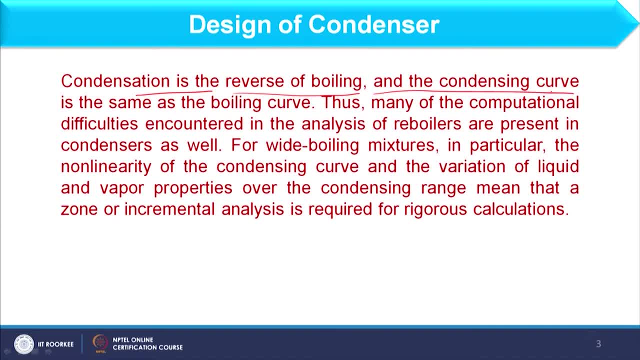 Okay, So you see, condensation is a reverse of boiling. okay, Boiling we generate vapor, and in condenser we generate liquid. Okay, Condensing curve is the same as the boiling curve. thus, many of the computational difficulties encountered in the analysis of reboilers are present in condenser as well, because both 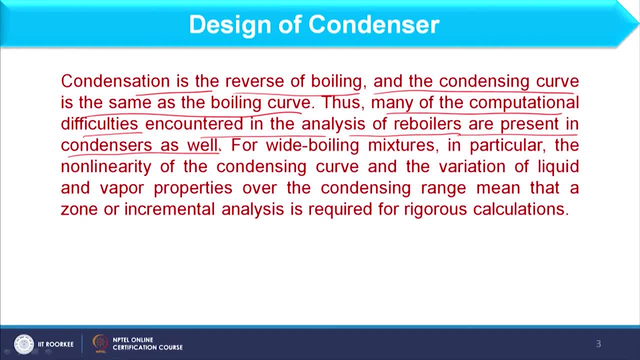 activity are just opposite to each other, right? if I consider reboiler and if I consider condenser? okay, So for wide boiling mixture in particular, the non-linear reaction, Okay. Okay, So the non-linearity of condensing vapor and the variation of liquid and vapor properties. 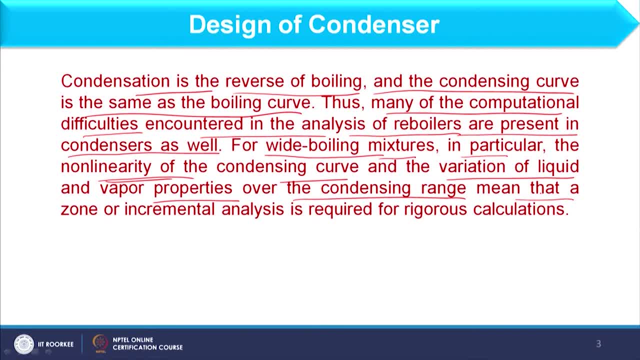 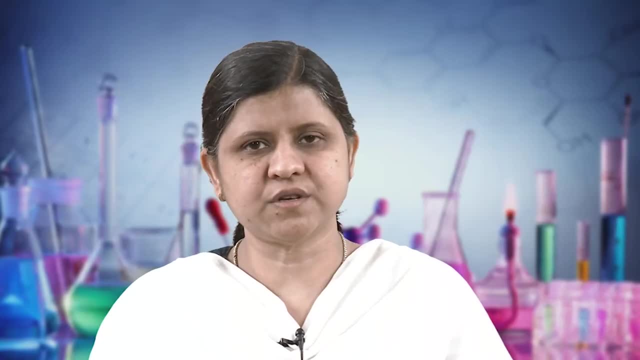 over the condensing range mean that a zone or incremental analysis is required for rigorous calculation. So you see, here we have considered reboiler and condenser just opposite to each other, and what difficulty we can obtain- Okay, Because it is not the easy method, because it is not an easy phenomena, and some rigorous 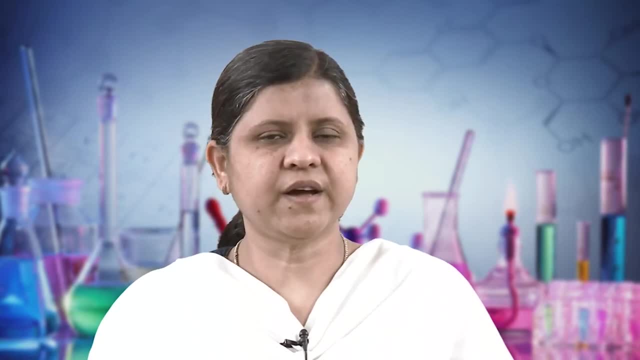 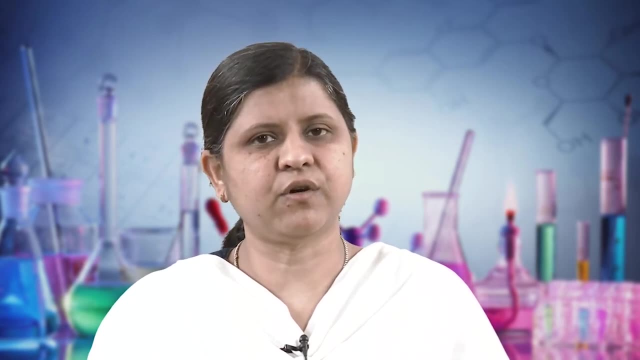 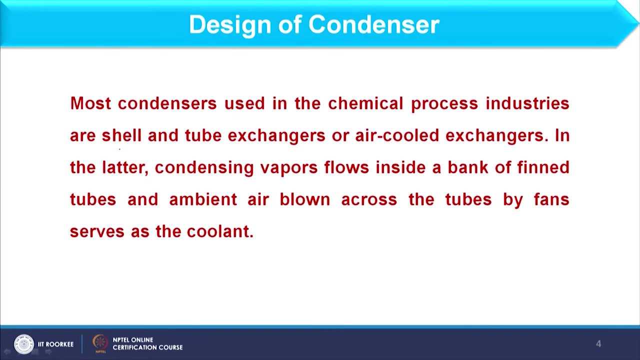 calculation should be required. okay, Why we require design of the condenser? because its use in chemical industry is extensive, which we have already discussed. okay Now, most of the condenser which are used in chemical plant are shell and tube type. Okay, 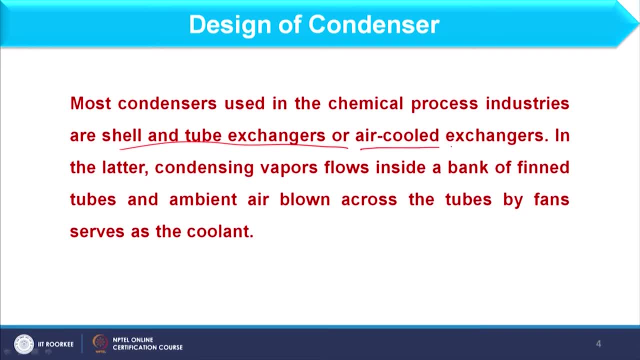 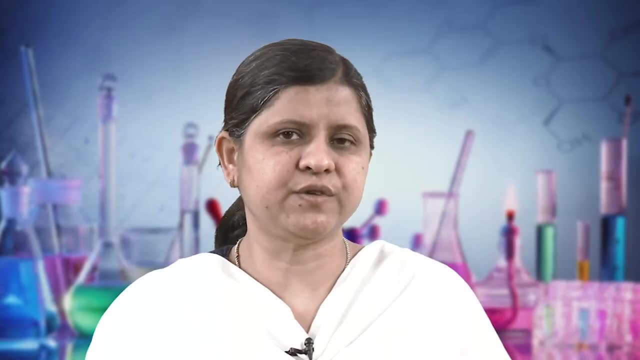 Okay, And in some cases, we also use air cooled exchangers. okay, So these are specifically shell and tube types, as well as air cooled exchanger. Air cooled exchanger: we have already discussed in detail when we have discussed classification of exchanger. okay. 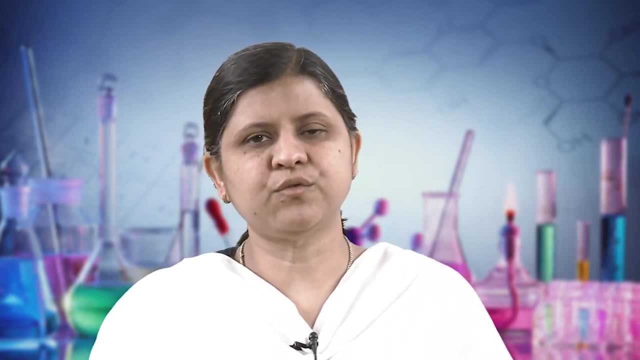 So that lecture you can refer to understand air cooled exchangers properly. Now what will happen with air cooled exchanger In copper tube? we have vapor which is cold, Okay. We have vapor which is to be condensed and over that in cross manner we inject air- okay. 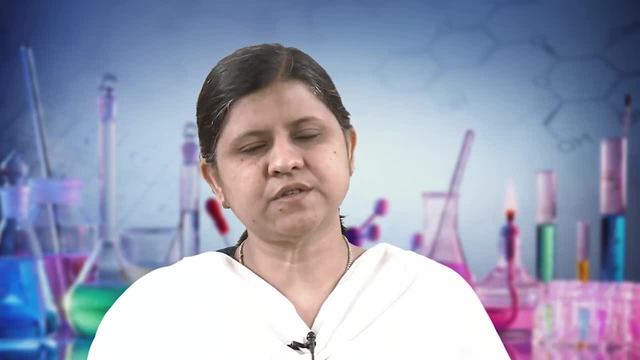 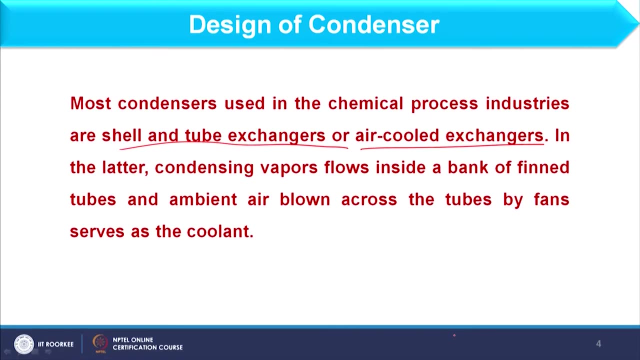 So instead of some cooling liquid media, we use air to condense the vapor. okay, So you can understand. in air cooled heat exchangers we usually use fan which is used as a coolant. We usually use fan in which air is used as a coolant. 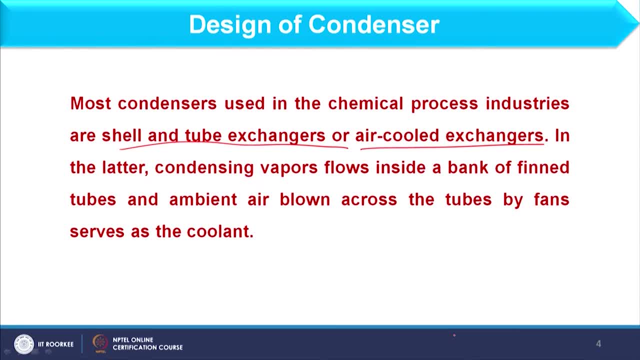 Instead of water in shell and tube heat exchanger. right. So what we can observe over here- that most of the exchangers are shell and tube type and apart from that, other type of exchangers are also used. but its use as condenser is. 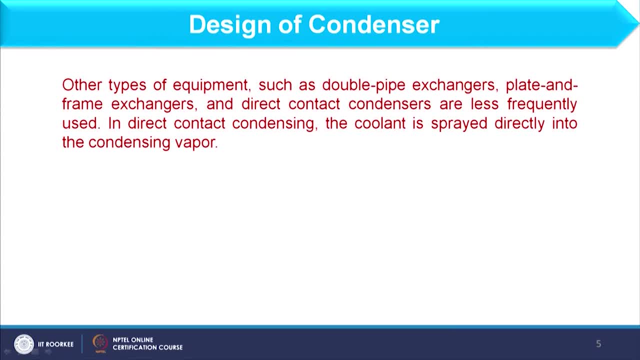 not significant, okay. However, other type of equipment such as double pipe heat exchanger, plate and frame exchanger and direct contact condenser are less common, Okay, less frequently used, however. it is used but use is not extensive. In direct contact, condensing coolant is sprayed directly into the condensing vapour. 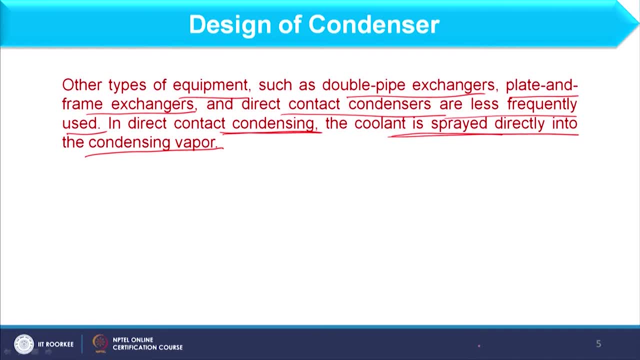 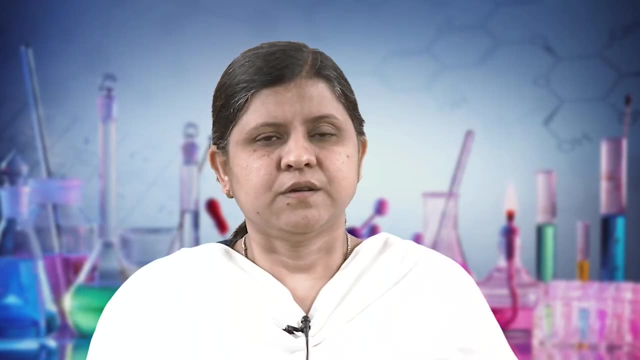 So you can understand that, apart from shell and tube heat exchanger, we have other exchangers also which are used as condenser, but not as frequently as shell and tube heat exchanger. So now discuss the types of shell and tube condenser, because we are going to design the 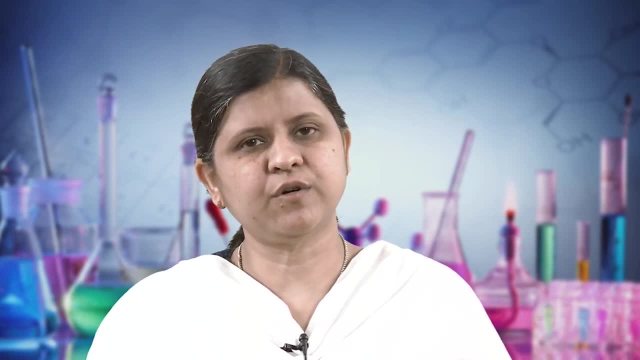 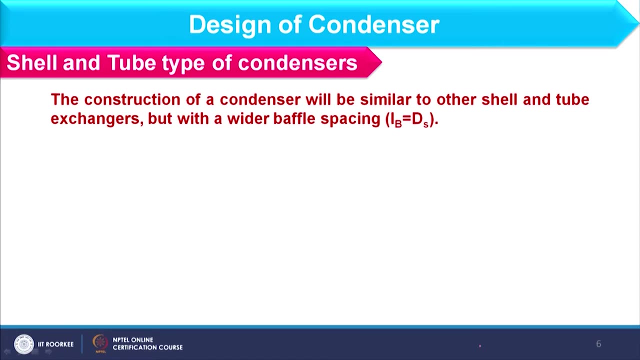 shell and tube condensers only. So we will discuss type of these condensers only. So if you focus on the construction of a condenser, It is similar to a condenser. So shell and tube heat exchanger, but with some modifications. 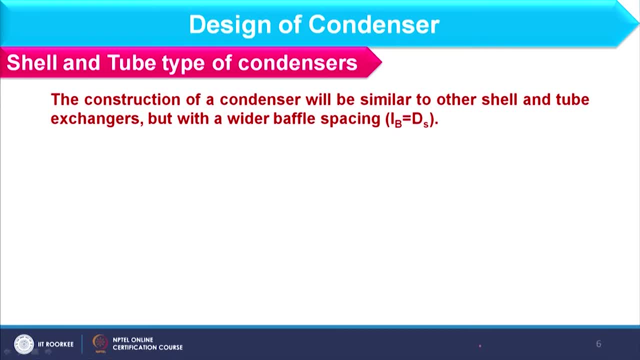 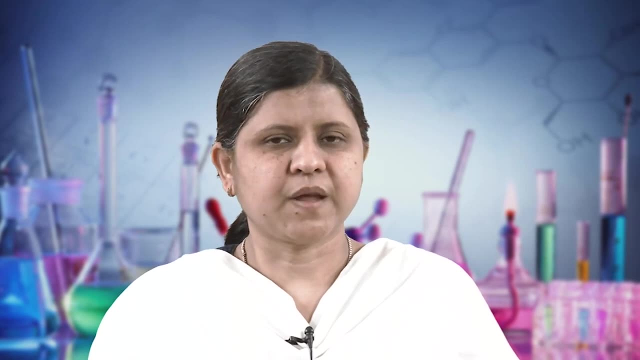 What is the modification Here? I am using wider baffle spacing, So in this case baffle spacing should be equal to ds. Now, here we will not follow the guideline for baffle spacing. that baffle spacing should be equal to 0.221 into shell dia. 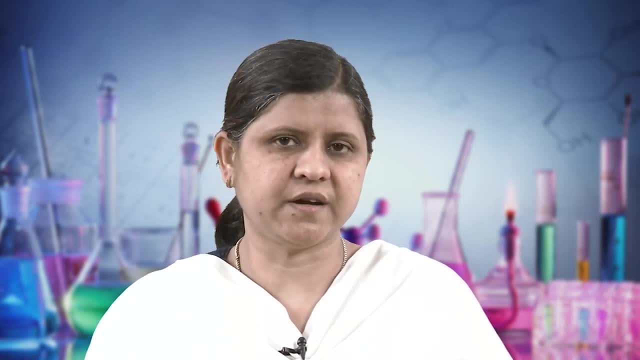 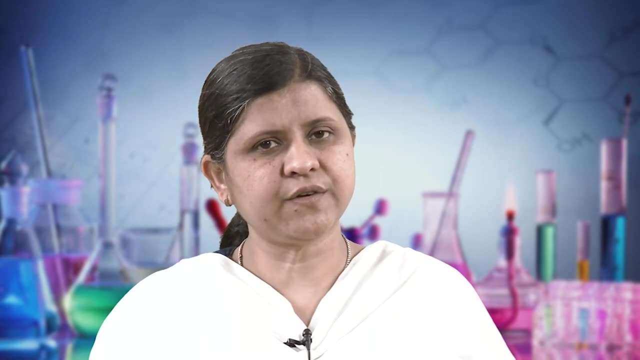 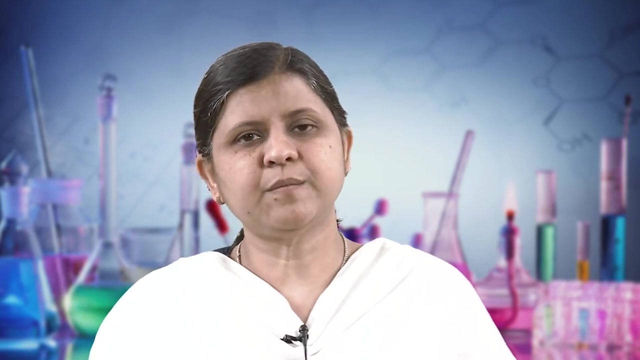 Here we will consider baffle spacing equal to shell dia When I am considering condensation in shell side. if condensation is in tube side, shell side should be designed normally okay, But here baffle spacing should be wider, and the reason is because we are considering vapour. 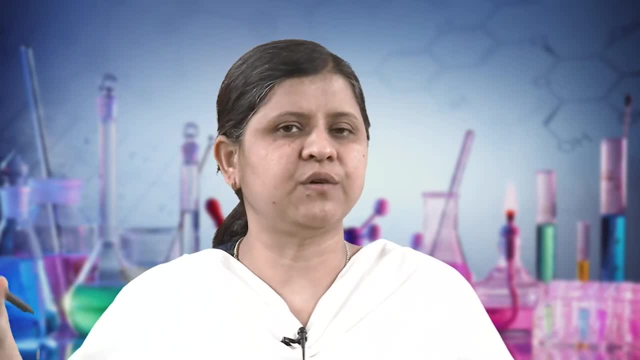 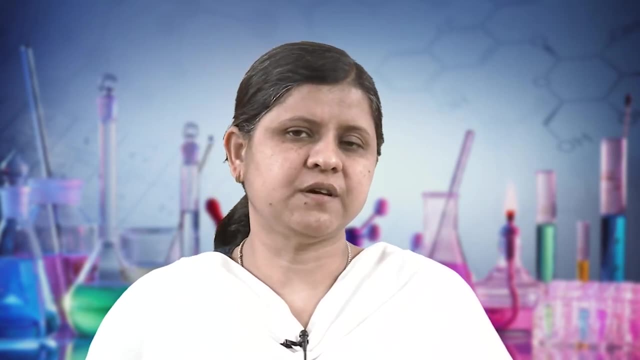 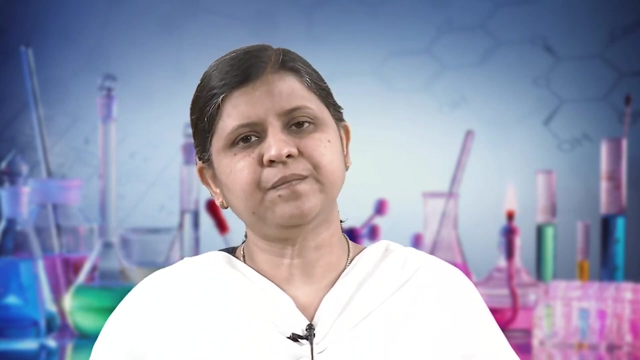 and vapour movement is not up and down, as usually we have. when the liquid stream is used in shell and tube. Okay, When liquid stream is used in shell and tube, exchanger right. So in this case, vapour move and vapour should require wider space to move. okay, and therefore, 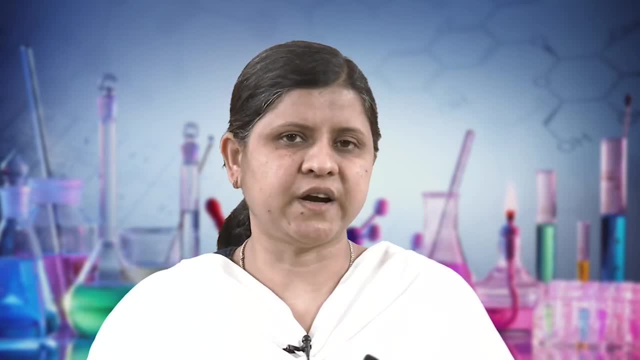 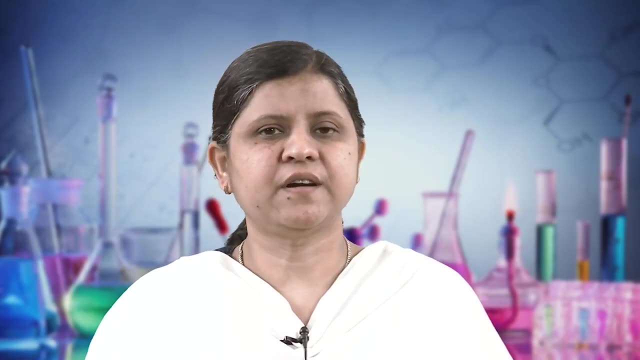 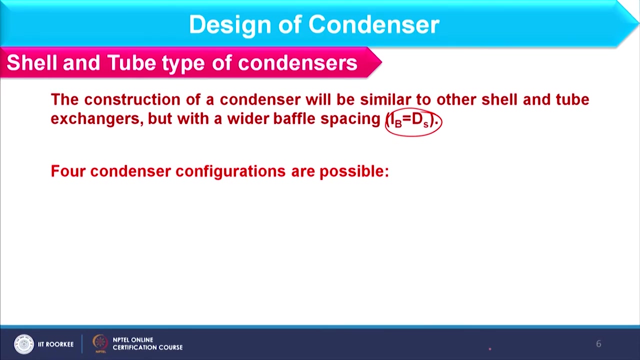 baffle spacing over here is equal to shell dia and that is very wide. I hope you can imagine that. So now let me classify the condenser, and usually we have four types of condenser, and these are shell and tube types. okay, And as far as classification is concerned, this is based on two factor. number one, based 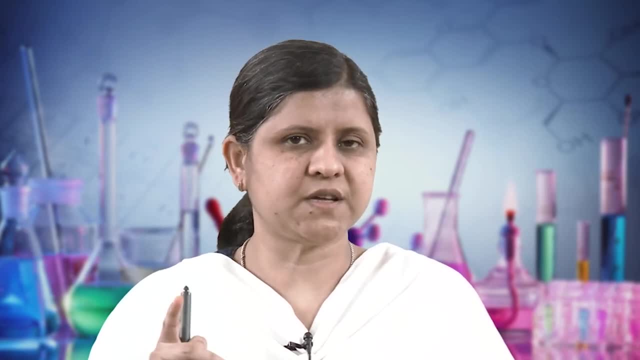 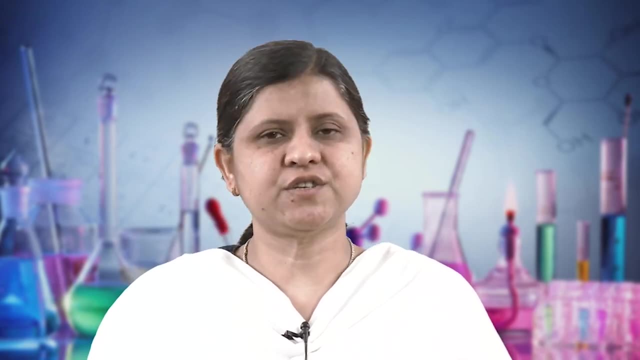 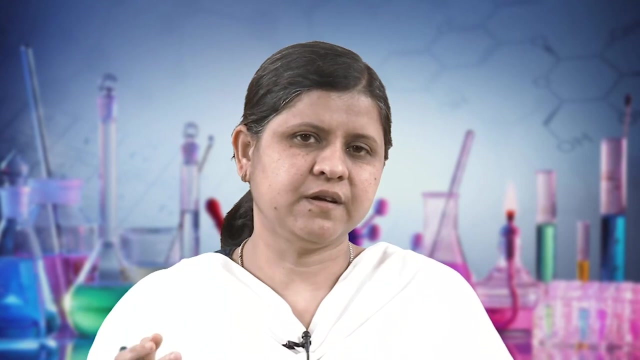 on orientation. okay, how it is placed. Second is where condensation is going on. okay, Now if I ask you where the condensation should be going on in shell and tube condenser, you have only two answer: either shell side or tube side. right, 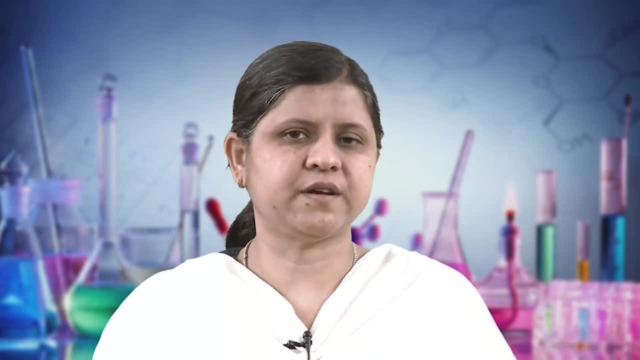 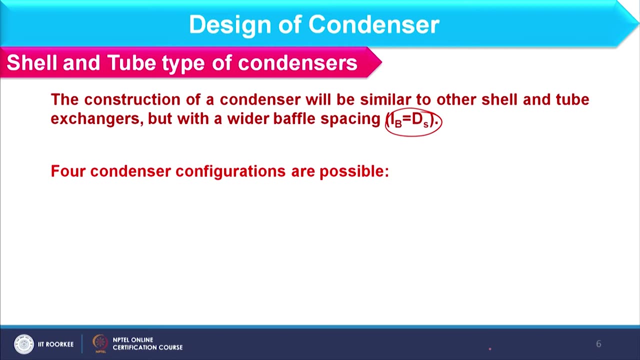 You have only two options, either shell side or tube side, right? Okay, Now if I ask you what is the orientation of condenser? So in that case you again should have two options. only one is vertical and second is horizontal, right? 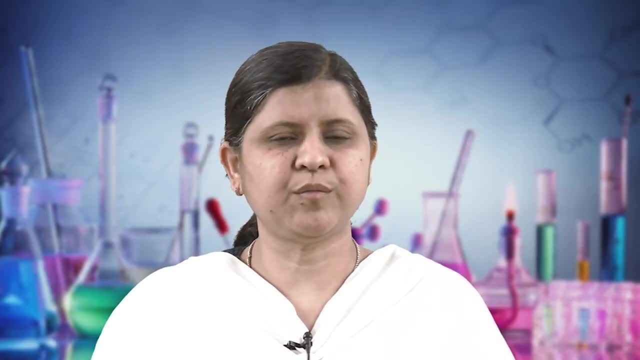 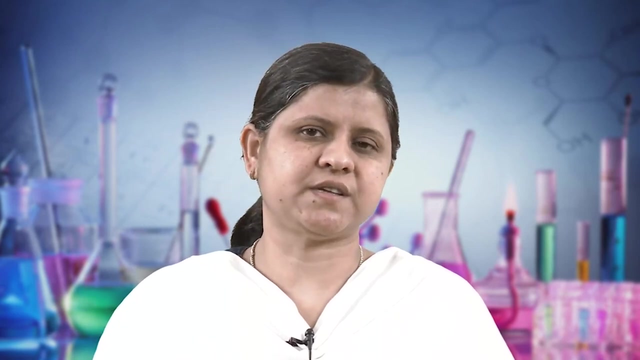 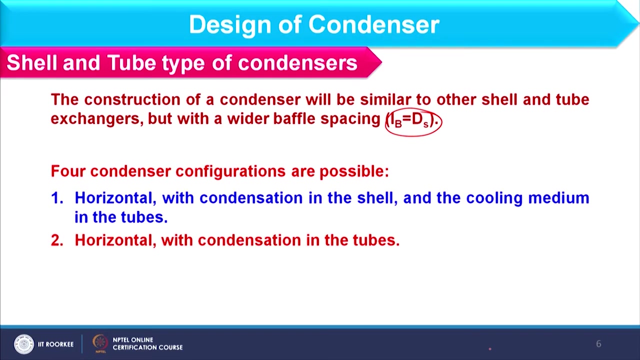 So only four condenser we can configure depending upon orientation and the side of condensation. And these four condensers are: horizontal condenser, where condensation is in shell side- okay, Okay, And cooling media is available in tube- okay. Second is horizontal condenser where condensation is in shell side. 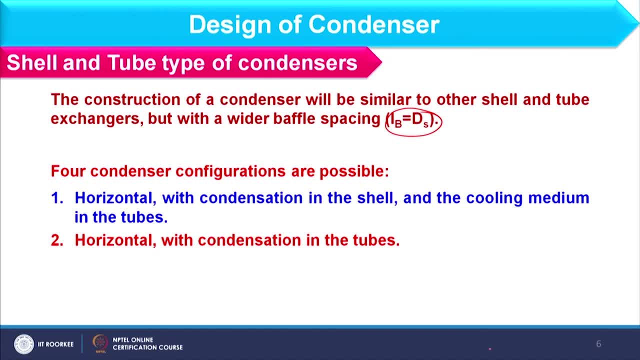 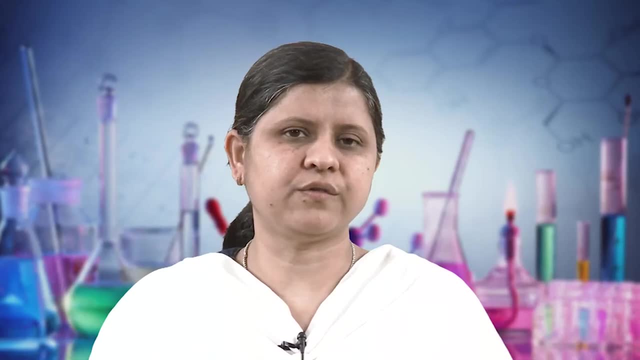 Second is horizontal condenser where condensation is in tube side- okay, In the similar line, vertical condenser where condensation is in shell side. and vertical condenser where condensation is in tube side. so we have four configuration, as you can observe. 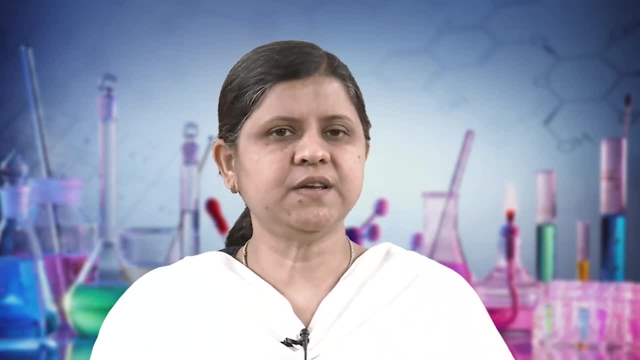 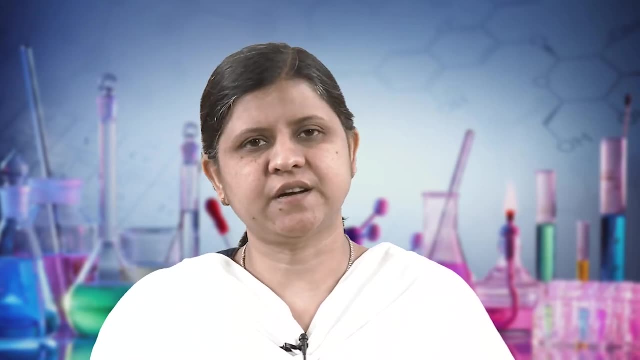 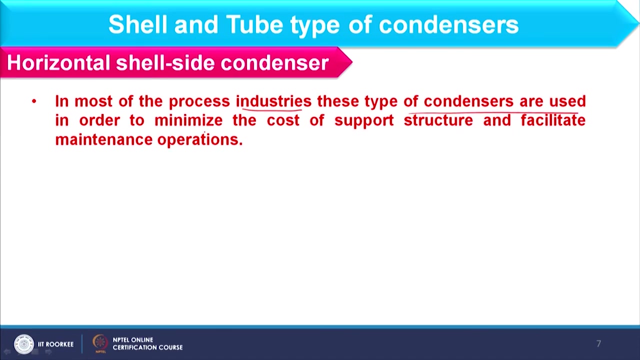 here. Okay, So now we will see each type of condenser in detail. So let us start with horizontal shell side condenser. So in most of the process industries, these type of condensers are used in order to minimize the cost of support structure and facilitate maintenance operations. okay, 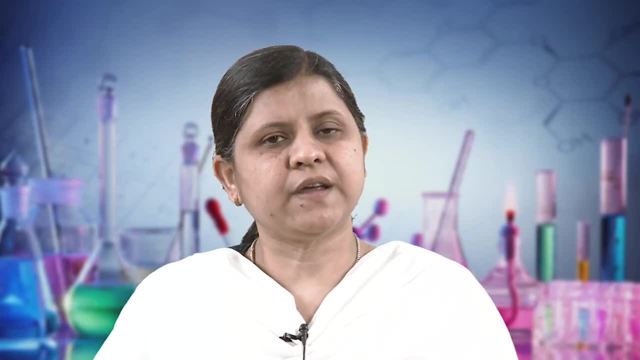 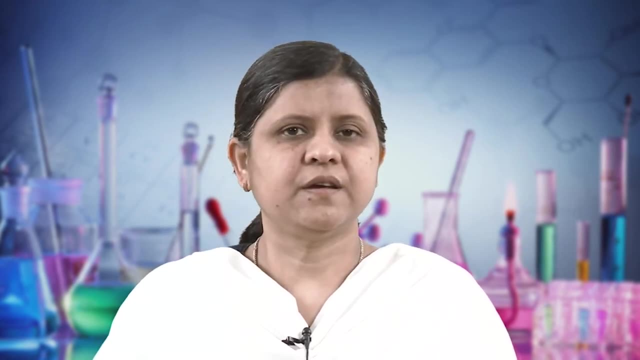 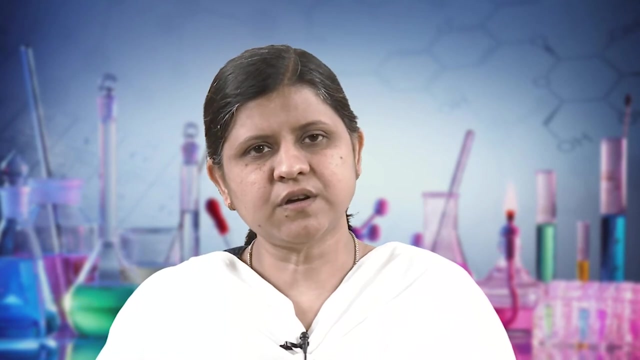 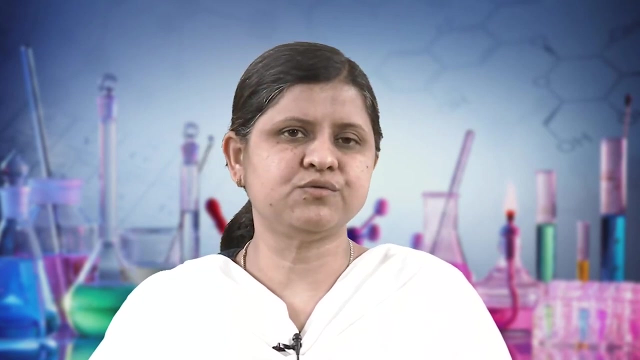 So what is the meaning of that? Your heat if your condenser is having larger duty? right, if your condenser has larger duty, it is better to place that condenser horizontally, because when I am placing the condenser horizontally I can provide better support in comparison to I am providing or I am placing large duty. 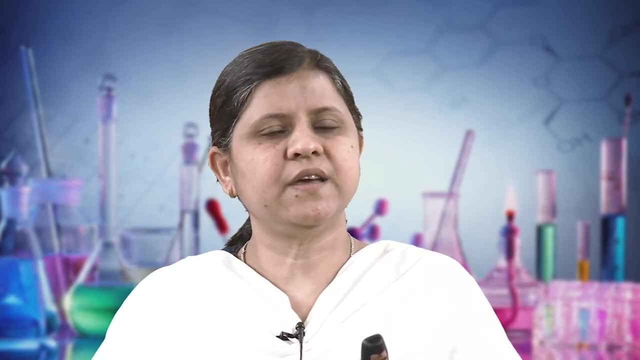 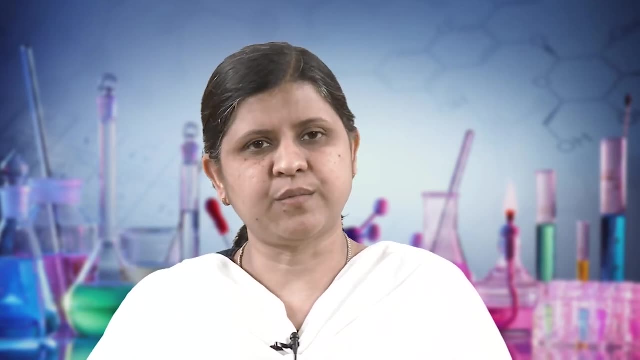 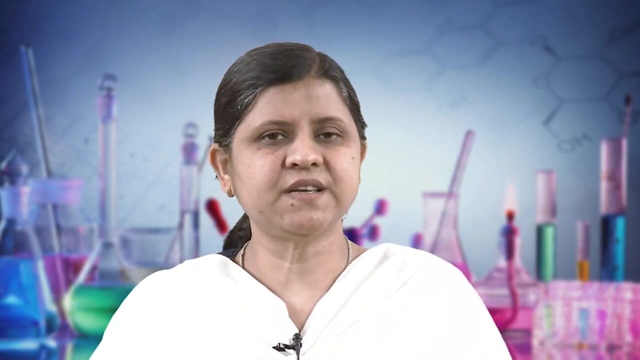 condenser vertically, Okay. So for vertical equipment, support structure is very important, okay, and that is not as easy as it is for horizontal condenser, right? So if duty of condenser is larger, we should place that condenser horizontally, okay? and 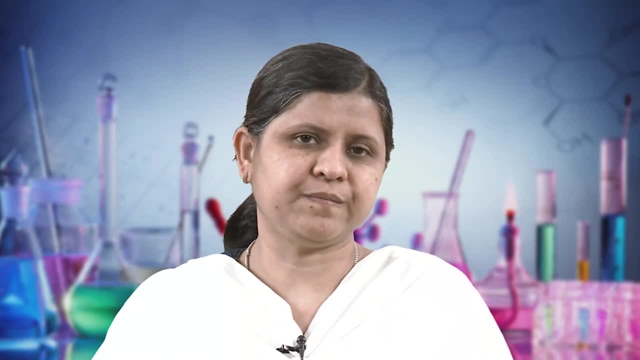 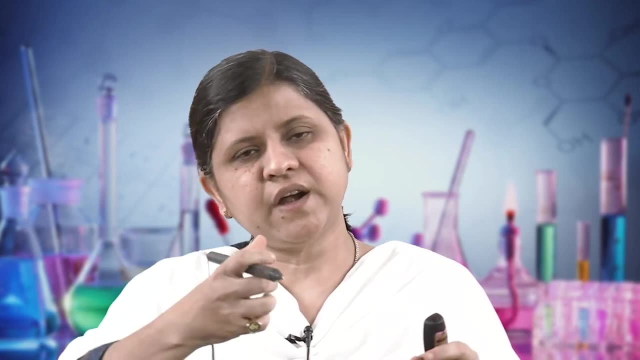 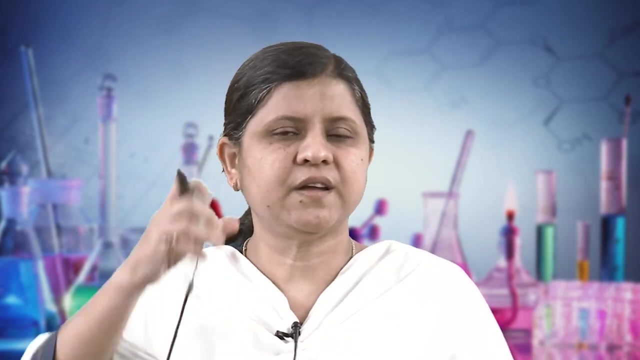 it will ease the maintenance problem also. How? Because when you have larger condenser and which is placed horizontally, you can take the bundle out very easily, right when it is placed horizontally. However, when it is placed vertically, the removal of bundle from shell is very difficult. 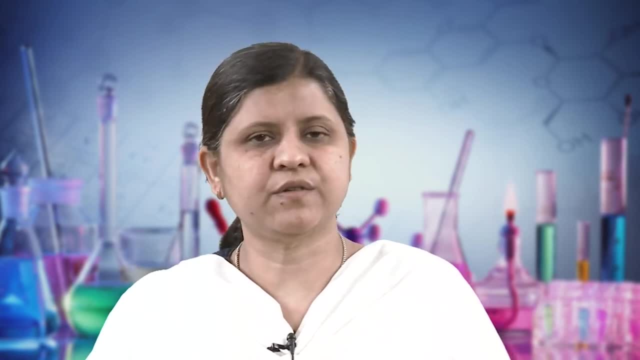 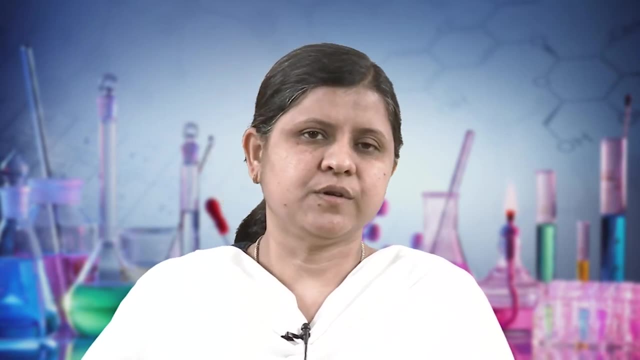 though that can be done, but when we compare the easiness of the maintenance, it is more easy in horizontal condenser. okay, So you should keep in mind. Okay, So keep in mind how you decide the placement of the condenser. 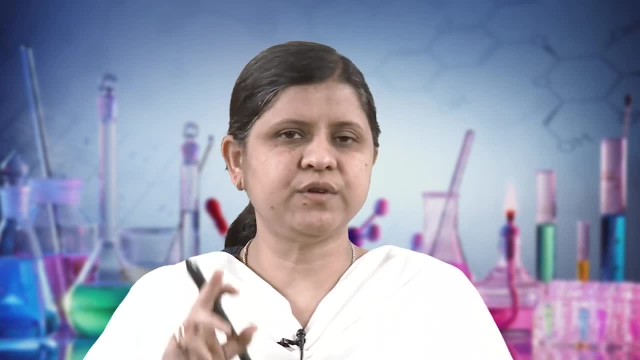 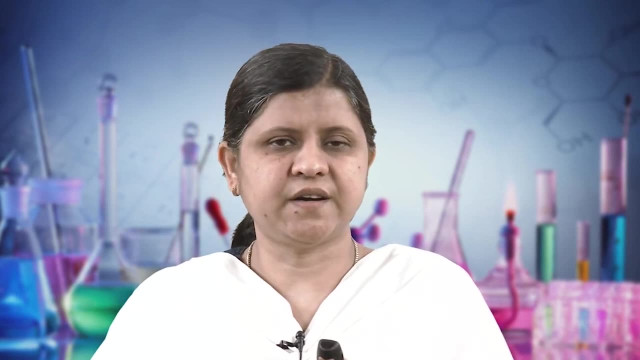 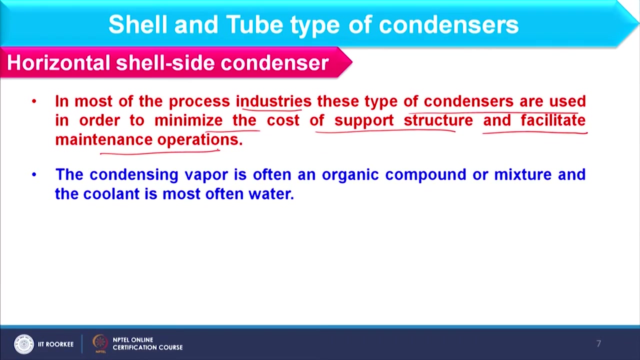 It will depend on larger duty. okay, If duty is small, you can place vertically, no problem, okay. So here we have horizontal shell side condenser, and if I am saying that shell side condenser, it means vapour should enter into shell side and the cooling media should enter into tube. 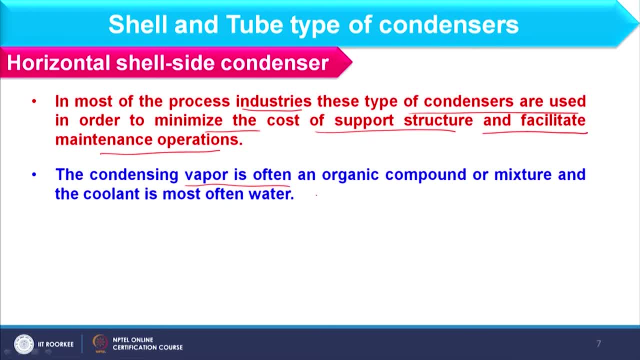 side. okay, So in this case, condensing vapour is often at the shell side. Okay, So condensing vapour is often an organic compound or a mixture and the coolant is most often as water. okay, So condensing vapour is most frequently placed in shell side. okay, and cooling media, which 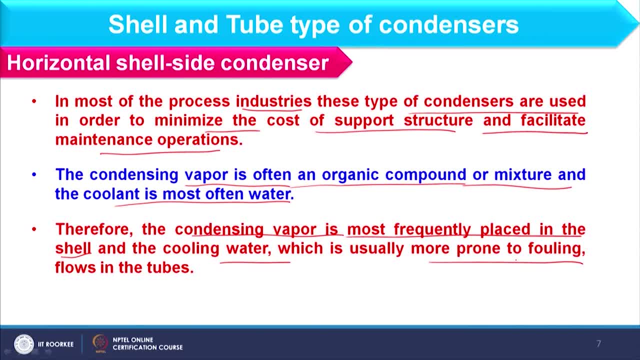 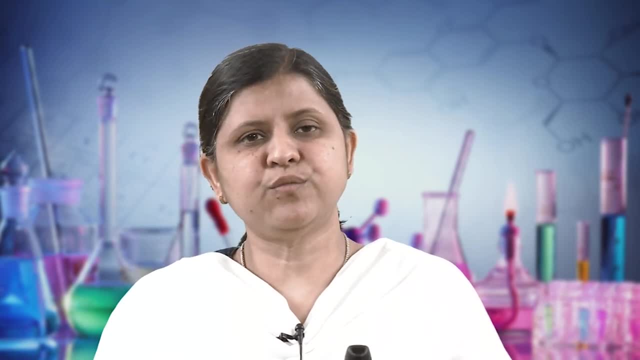 is, the water is usually more prone to fouling and therefore it should be allocated to tube side. okay. So shell side condensation vapour should enter into shell side, right? So condensing vapour: Okay. So now discuss few more points about horizontal shell side condenser, and here we usually consider: 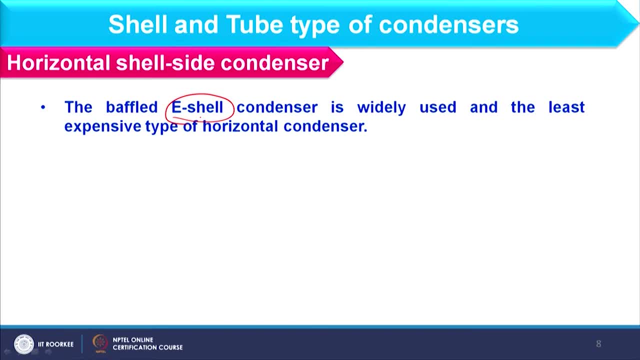 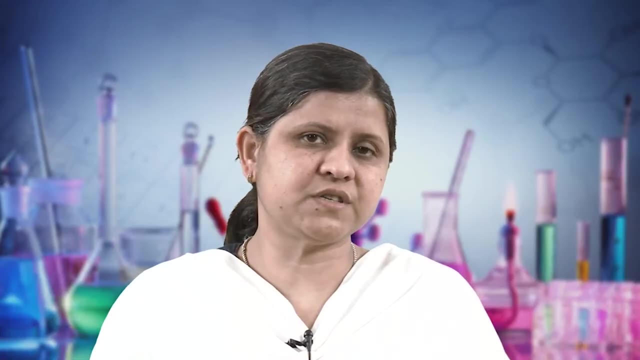 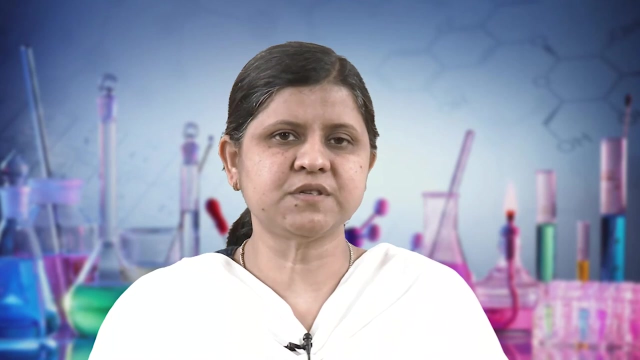 E shell. okay, So TEMA E shell is considered over here and it is widely used in a condenser and the least expensive type of horizontal condenser. So that you can understand, because TEMA E is the simplest type of shell. TEMA E is the simplest type of shell, so that becomes inexpensive, also in comparison to 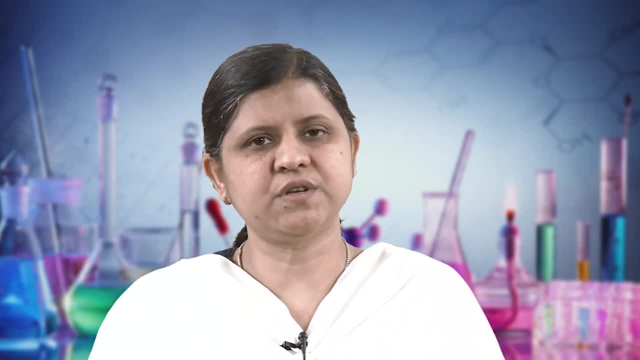 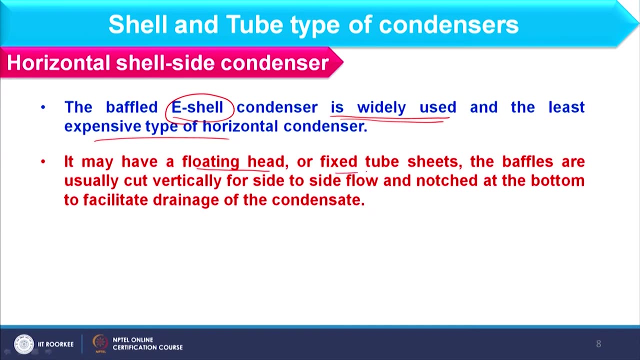 others okay and therefore it is widely used in condenser. Next is it may have floating head or fixed tube sheet, and baffles are usually cut vertically for side to side flow and notched at the bottom to facilitate drainage of the condensate. 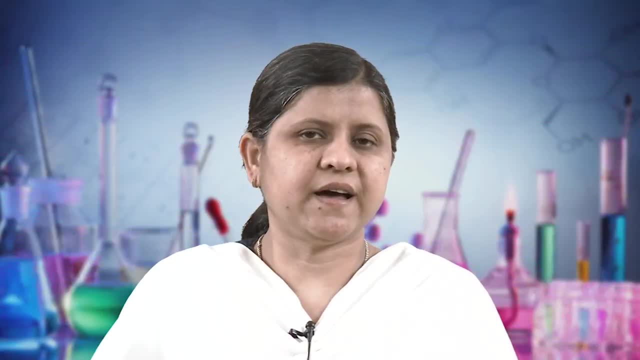 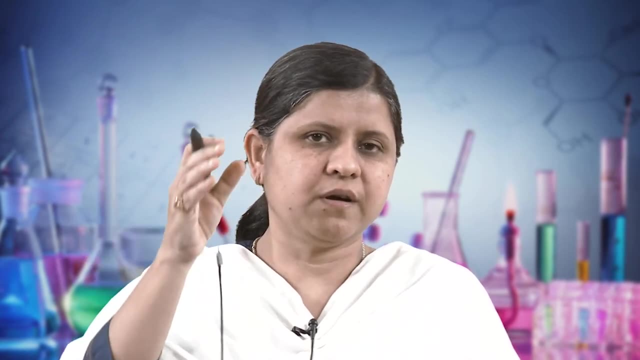 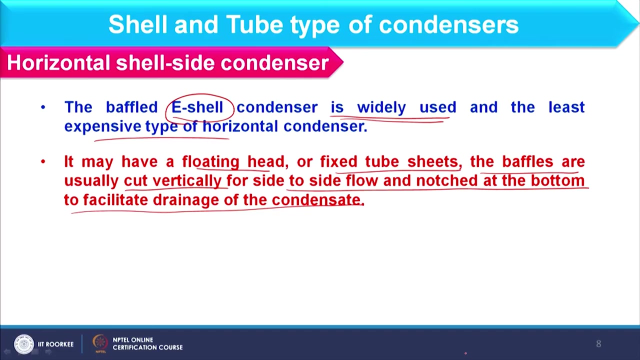 okay. Now let us consider this as when I am having a condenser in shell side. okay, So what will happen at top of the tube? condensate continuously form and moves downward right, So at the bottom, condensate will be collected. okay. 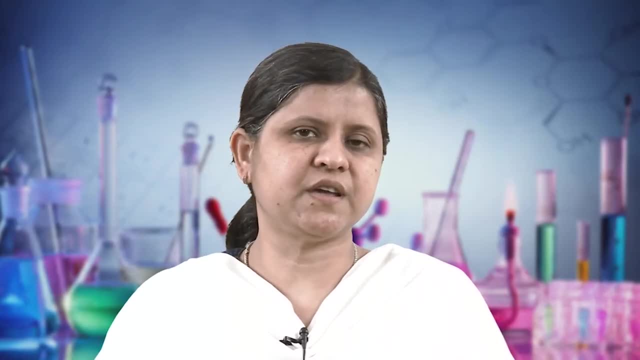 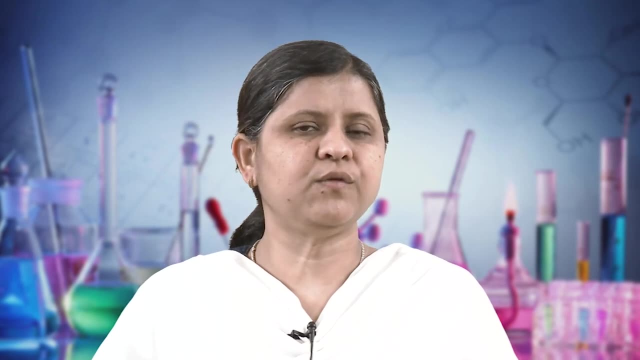 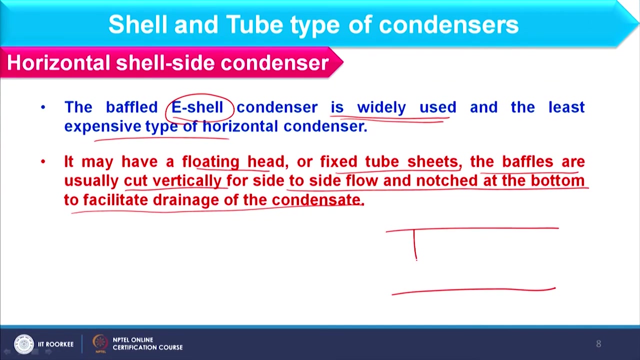 Now, in such type of condenser where condensation is taking place in shell side, we usually have vertical cut in baffle. okay, Till now what you have seen As far as baffle is concerned, usually we have this type of baffles, right. 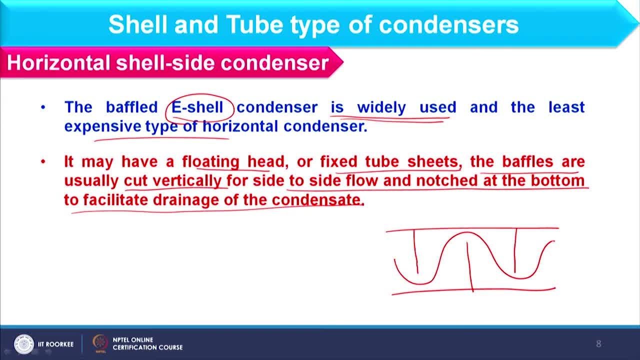 So movement of liquid is like this: okay, So we can consider this type of movement in liquid. However, when I am considering vapour, okay, vapour has lesser density in comparison to liquid, so it will never come down. okay, It will occupy the baffle. 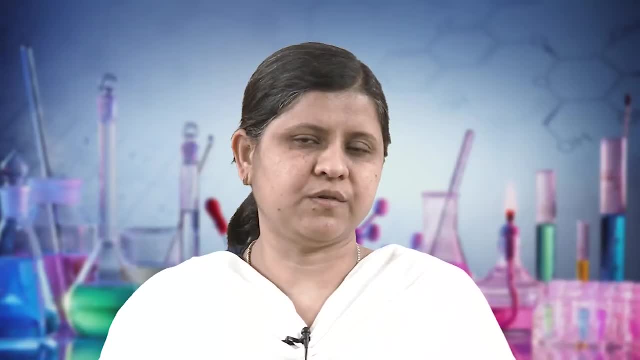 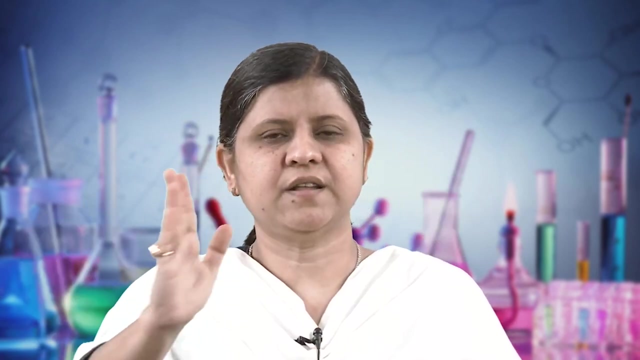 So it will never come down. okay, It will occupy the space, but it will not come down, okay. So in that case, instead of horizontal cut, we usually consider vertical cut, so that vapour can move like this. okay, I hope it is clear to you. vapour should move like this, okay, not like this, okay, as I 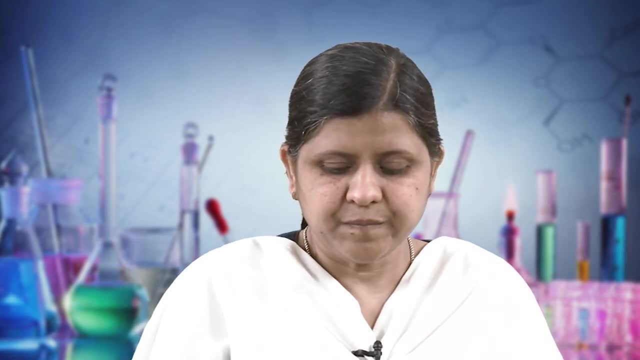 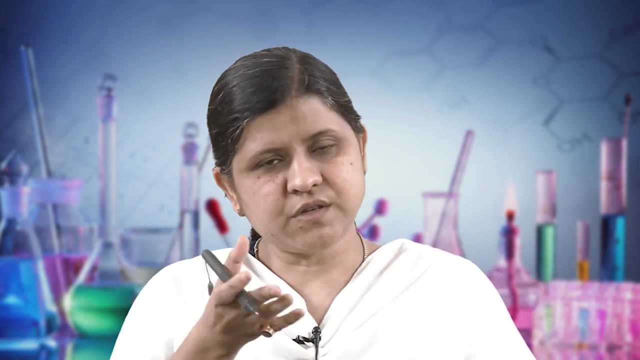 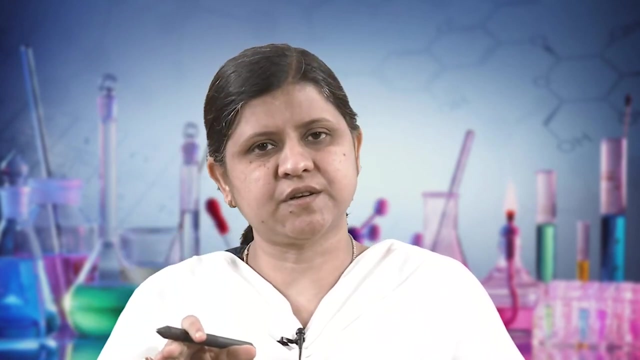 have just shown. So in this case, usually vertical cut is placed in baffle and it looks like this: Okay, Now what will happen? because horizontal cut is not there. so whatever condensate is collected at the bottom, it will remain in the exchanger. okay, it will remain in the condenser. 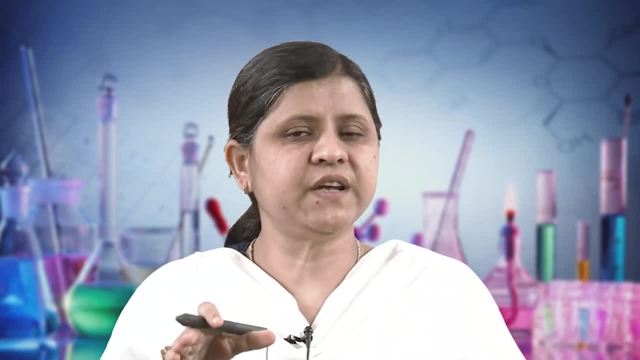 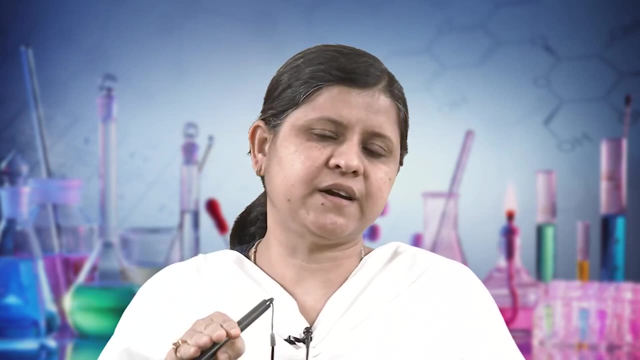 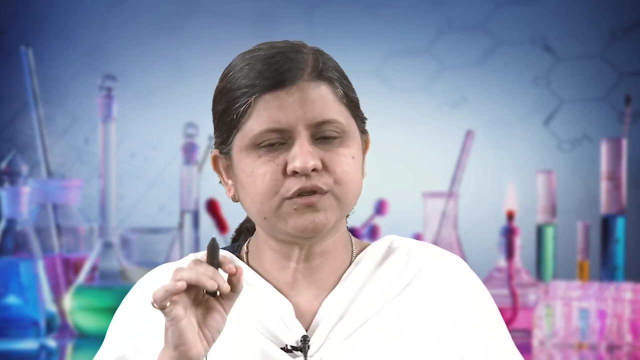 Now, what will happen when the condensate will be available in shell side? what will happen? some of the tubes will be merged in that condensate. I hope you understand, okay. and when it will be merged in a condensate, those tubes will. 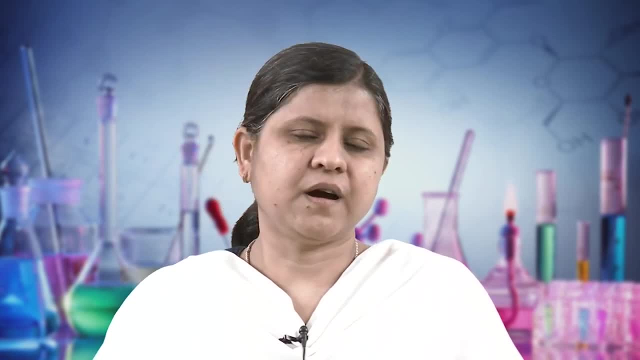 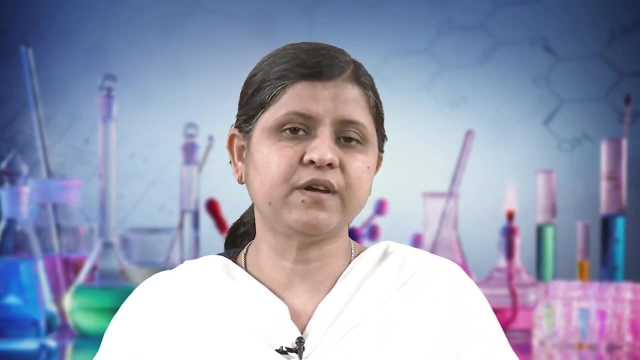 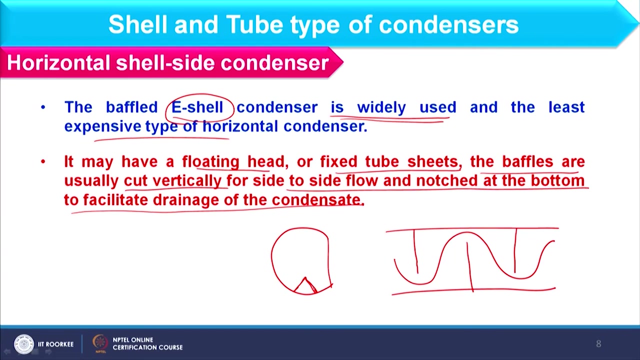 not participate in condensation process anymore until unless condensate should not be removed. So how we can remove the condensate when baffles are having vertical cut For that, we usually place a V notch- okay, V notch- at the bottom of the condensate and 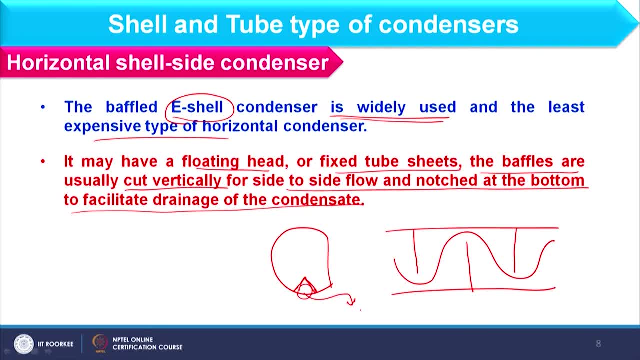 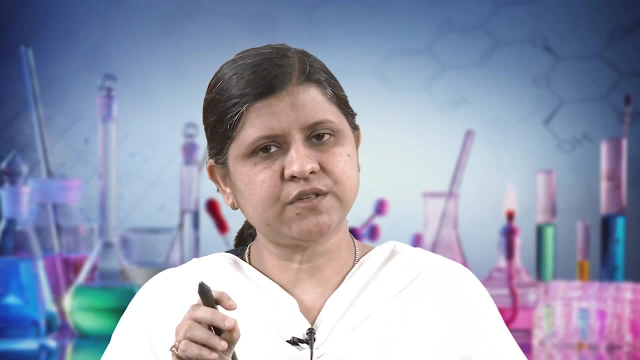 from this open space. condensate is continuously removing right so we can have removal of the condensate. Okay, So you should keep in mind horizontal shell side condenser. vertical cut baffle is used with a notch at the bottom for drainage of the condensate right. 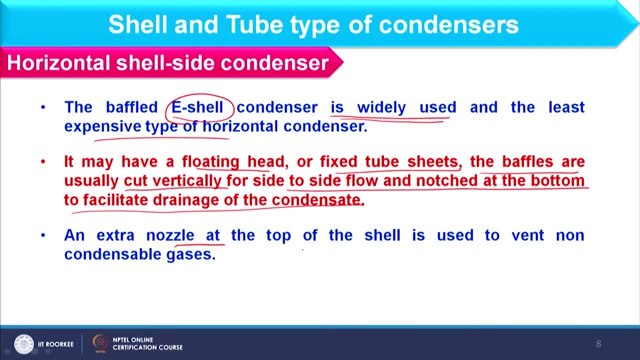 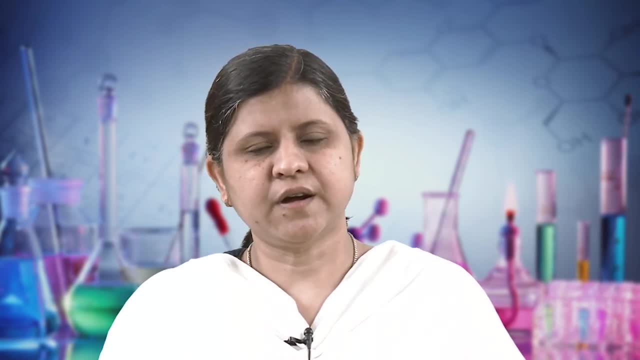 And further. we can have one extra nozzle at the top of the shell, which is used as a vent to remove non-condensable gases. okay, So let me explain this further with the help of schematic. Okay. So here we have the condenser, okay, and here vapour is entering into the shell side and 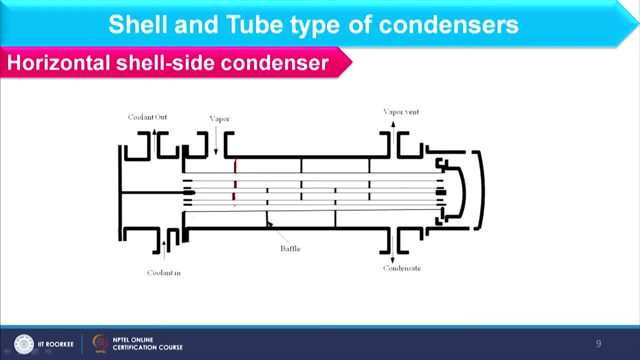 if you see, in this case, baffle should be like this: okay, baffle should be like this: okay, because we have vertical cut in baffles, okay. So vapour is entering into the shell side and from here at the bottom we have condensate. 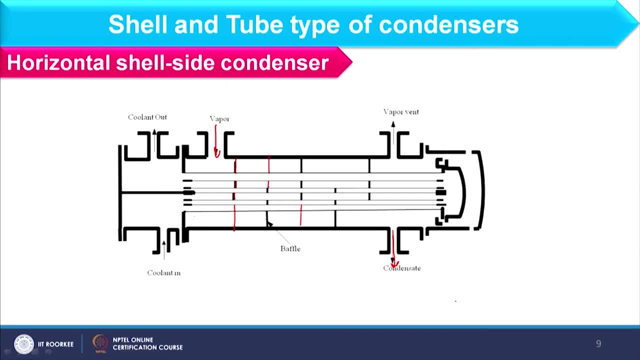 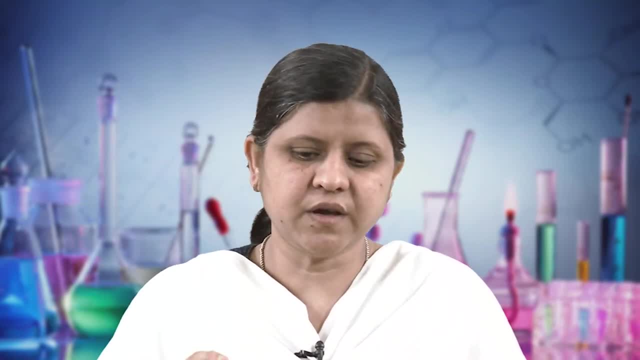 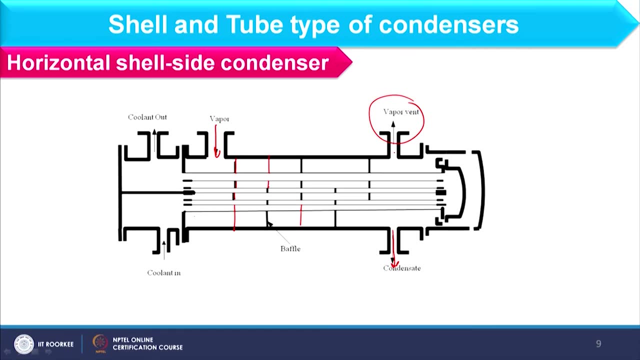 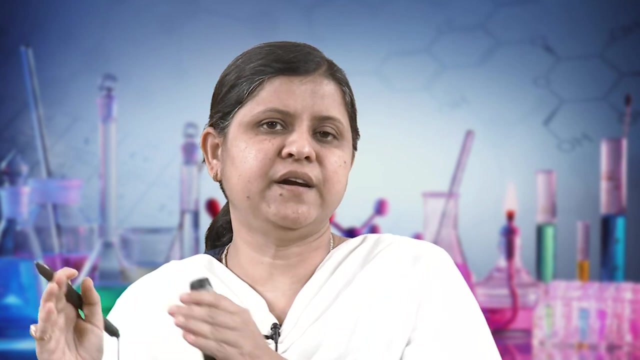 removal continuously. okay, Now, what we have discussed previously, that it has one extra nozzle and that we call as vent. okay, so that you can see, here I am having a vent which is just at the end of the exchanger. okay, If vapour is entering from one end at another end, vent should be there. okay, 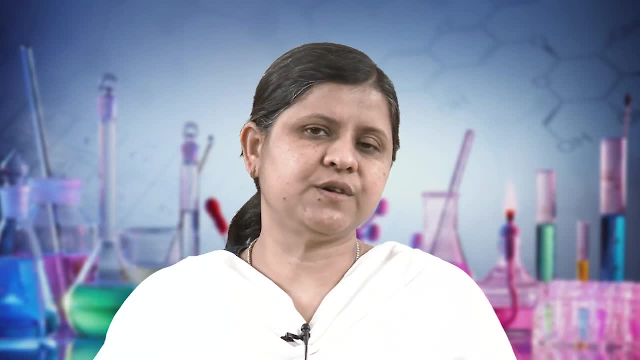 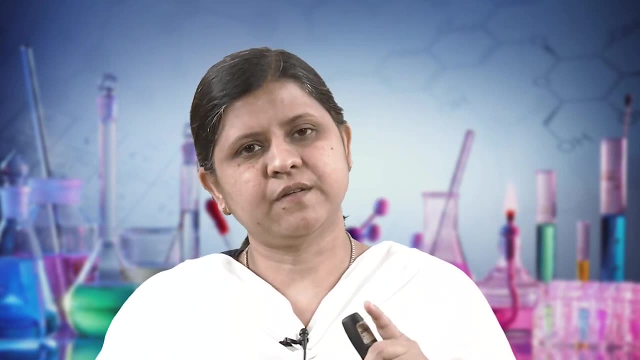 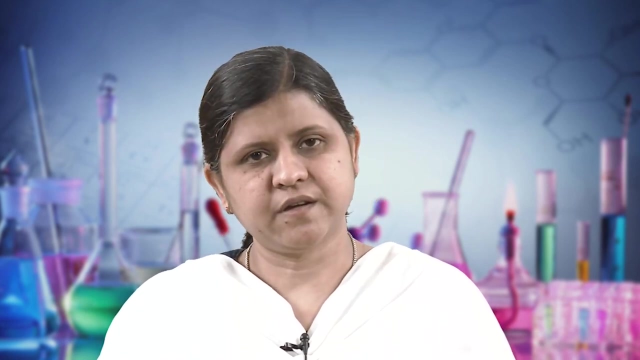 So what is the purpose of this vent? Okay, Now I ask you that if operation is not going on in a condenser, okay, then what will happen? The condenser will remain empty? The answer is no, because air must be there, right, and you understand that air is non-condensable. 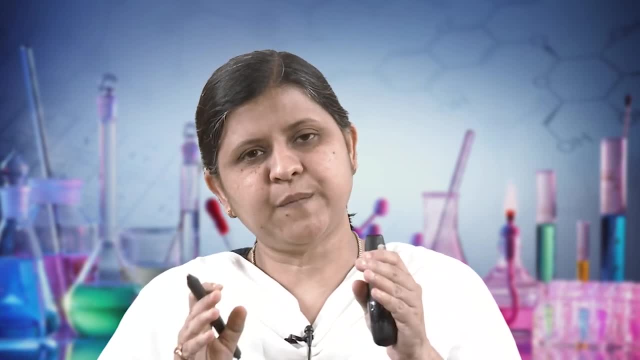 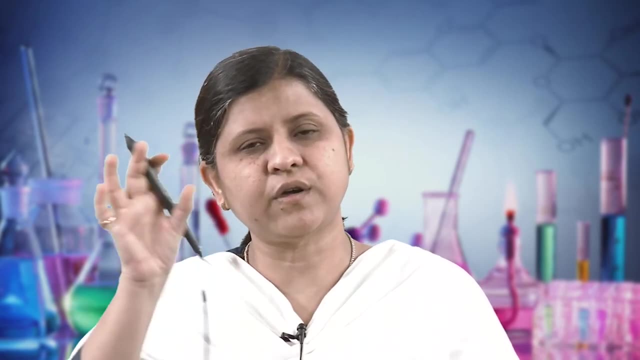 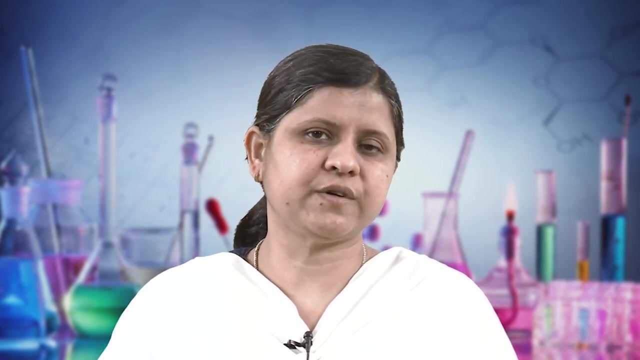 gas in nature. okay. Now what will happen when the vapour will enter into the condenser and air will not be removed? Okay, The vapour will occupy some of the space in condenser. okay, which will reduce the heat transfer area which is available for condensation. 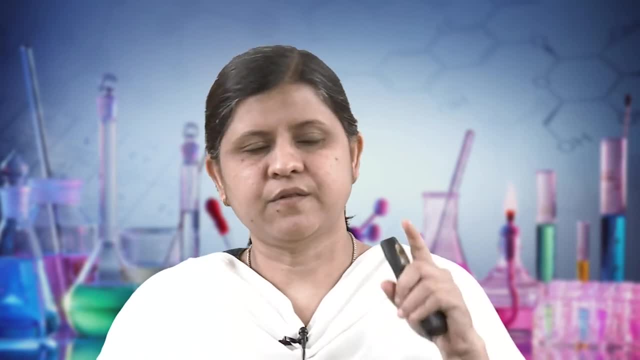 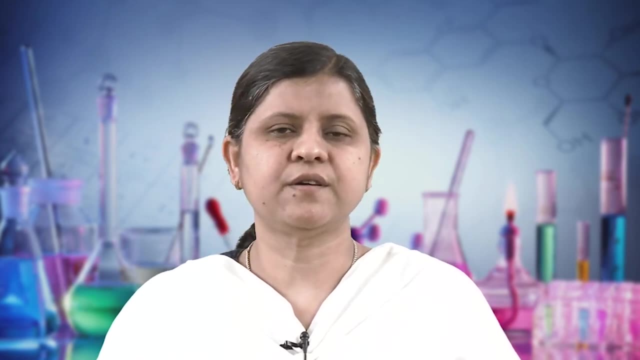 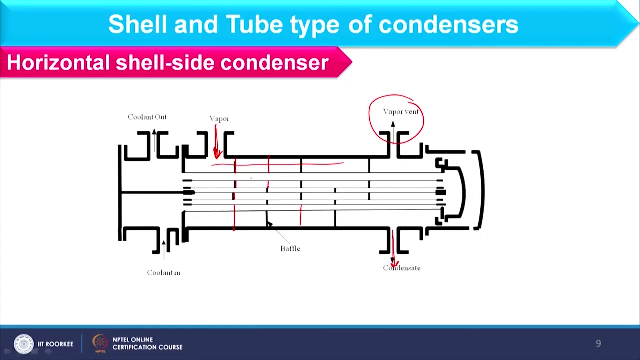 So when I am using the vapour, okay, when I am using the vapour in such equipment, we must have one extra valve and that we call as vent. okay, Now what will happen from this side when vapour is entering it? is continuously moving in. 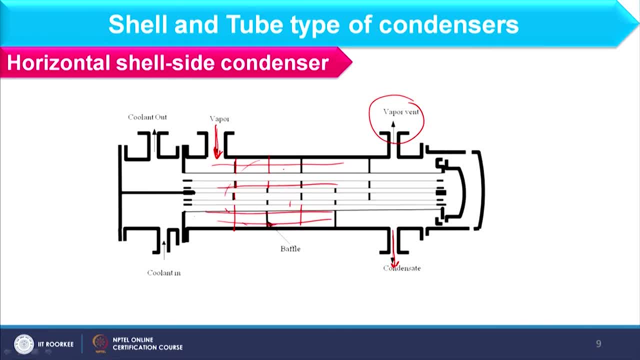 this side right. So whatever air is available in this, it will move to this direction. okay, because from back side vapour is coming Now as we increase. now as we open this valve, at the same time vent valve should also be opened, okay. 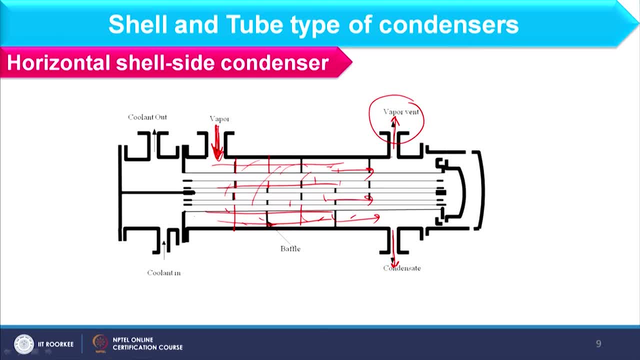 So, as vapour will keep on entering from this, Okay, So non-condensable gases will keep on leaving from vent side. Now what will happen after, when this vapour occupies the whole space? it means that non-condensable gases have been removed from the system, okay. 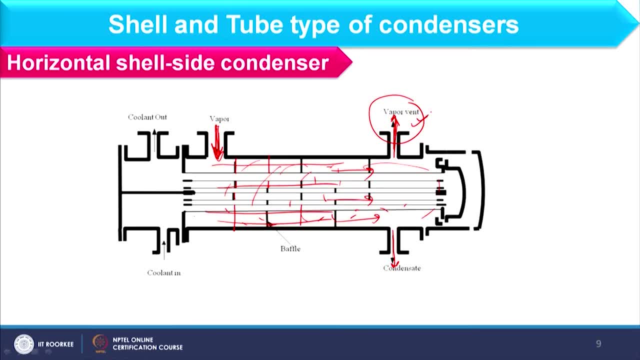 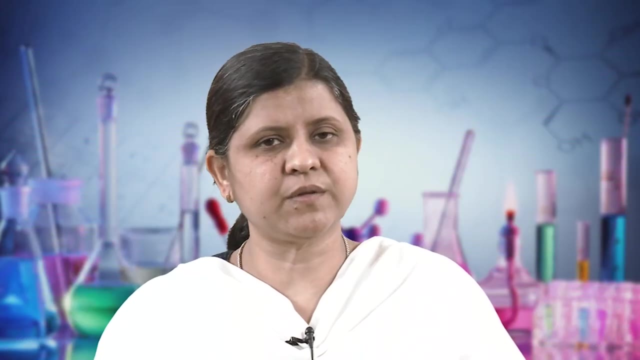 And how we will ensure that That, when this valve will keep on, when this valve remains, when this valve remains, when this valve remains open, after sometime, whatever vapour is entering, it will start moving from this nozzle or from this valve. So, in that case, when vapour is starting now, in this case, when vapour starts exiting from 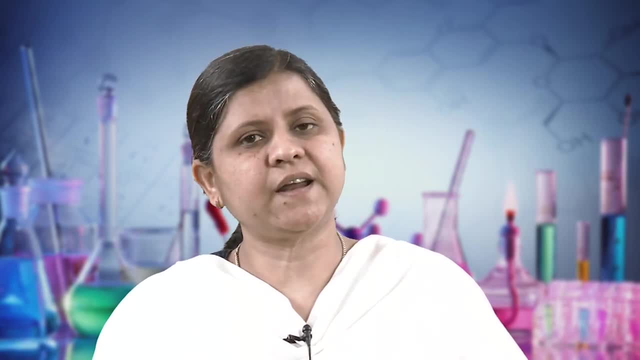 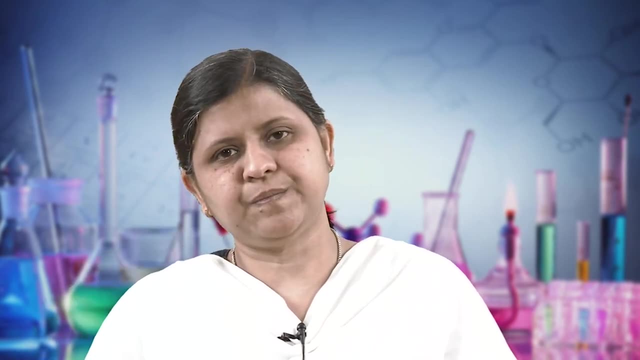 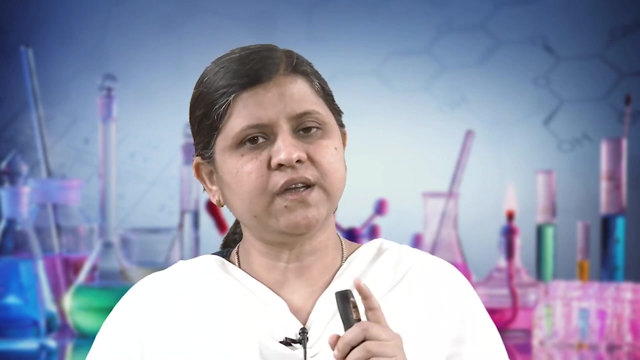 the nozzle or from the vent valve, we can say that air is completely removed from the system and at that time we close that vent right. So in this way we remove all non-condensable gases from the condenser. Even it is not used only in condenser: wherever I am using vapour either, it is condenser. 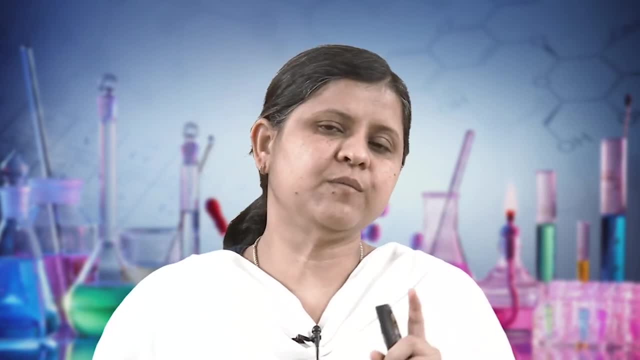 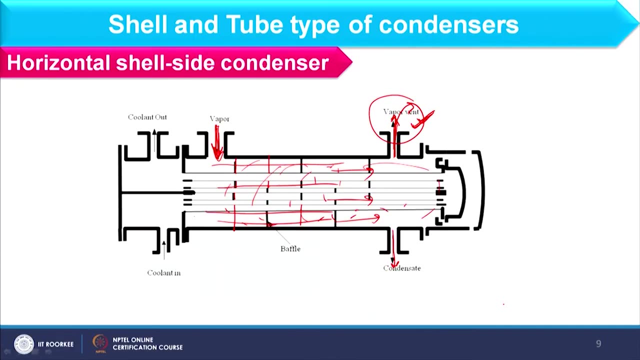 it is reboiler. it is a boiler wherever I am using vapour or steam. in that case, we consider vent as well, okay? And second point is what we do with condenser? Okay, Okay. So what we do with this condensate? okay, 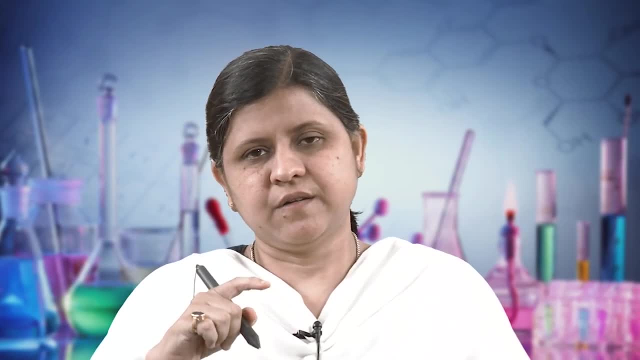 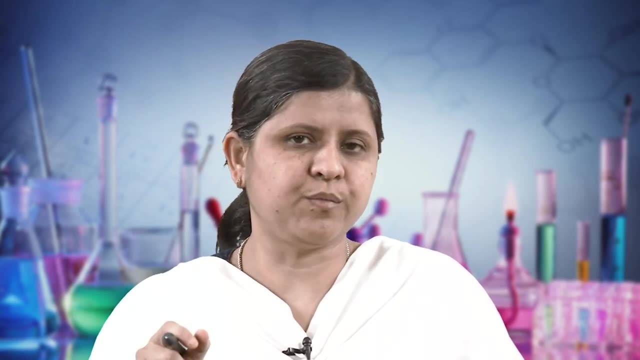 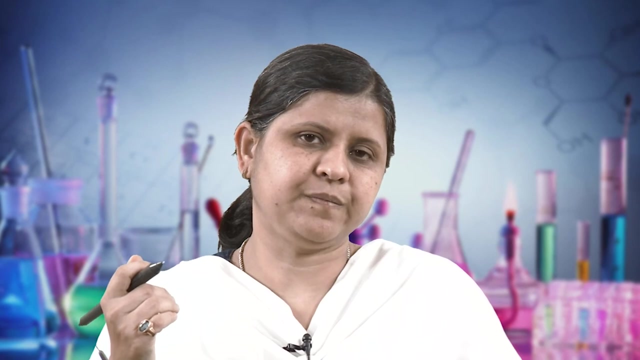 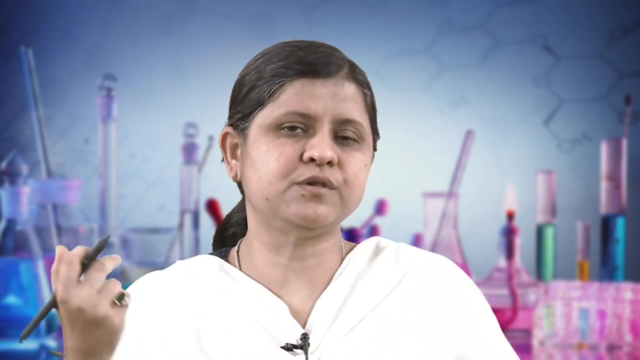 Because when condensate will exit, when the valve of condensate remains open, okay- and when the operation is going on, condensate will keep on exiting from the system right, And because vapour is also there, so there are chances that vapour should also exit the 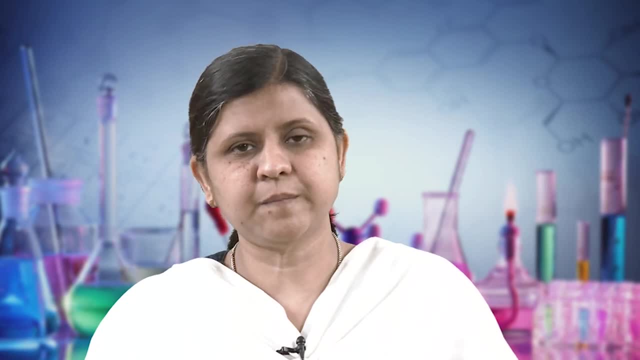 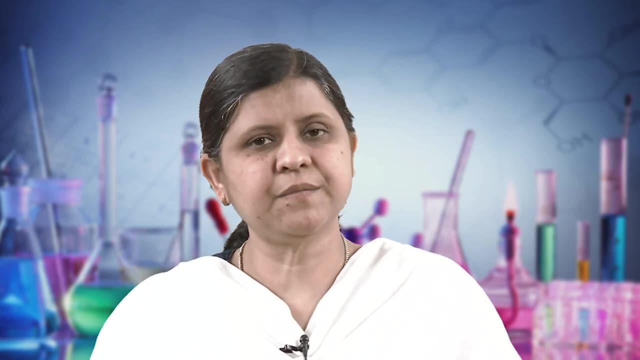 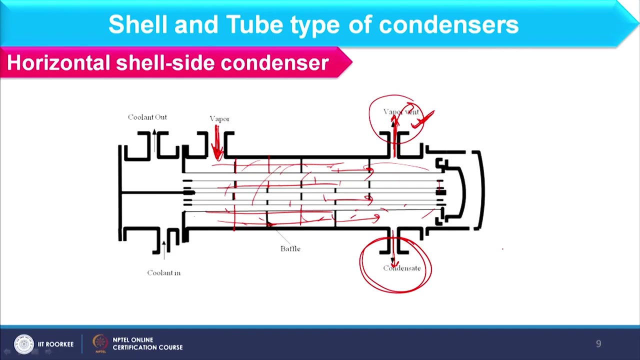 system from condensate. Okay, So to stop vapour into the system and to let condensate exit the system, we use another assembly, which we call as steam trap, which basically traps the steam or vapour. okay, So in that case, when I consider, let us say, condensate is exiting from here along with 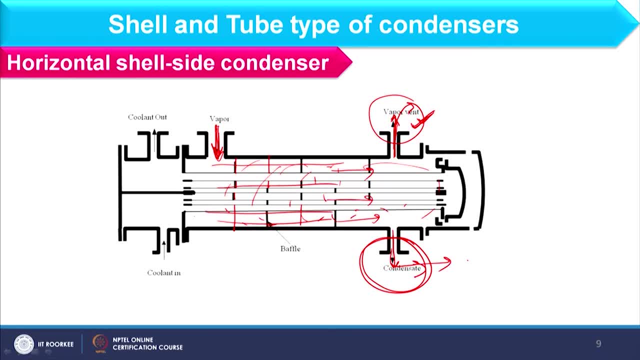 vapour, because you cannot stop vapour to moving out. okay, So it will enter into the system. Okay, So it will enter into this steam trap, which is this type of structure. okay, And from here we have the exit nozzle for condensate. 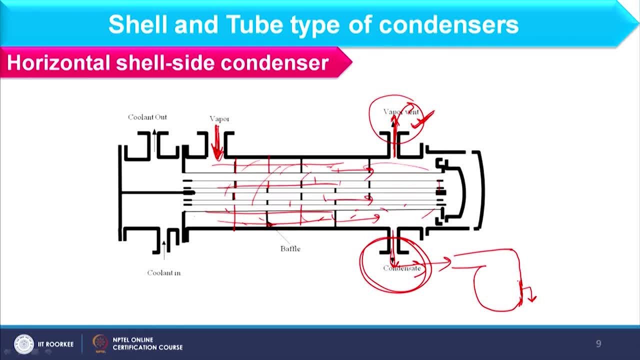 Now what will happen? usually this is closed with a valve and that valve is connected with a balloon. okay, This type of balloon is there and when I am having vapour and liquid mixture which is entering into this, So we have vapour as well as condensate. 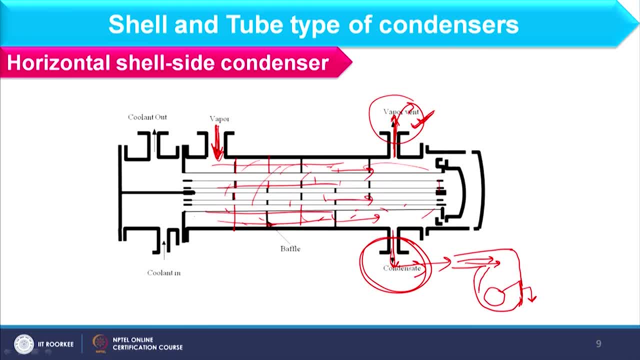 So what will happen? because of the density difference, condensate settles down right, So condensate will start filling this space. okay, So as condensate will start filling this space, it will let this balloon to move up, okay. 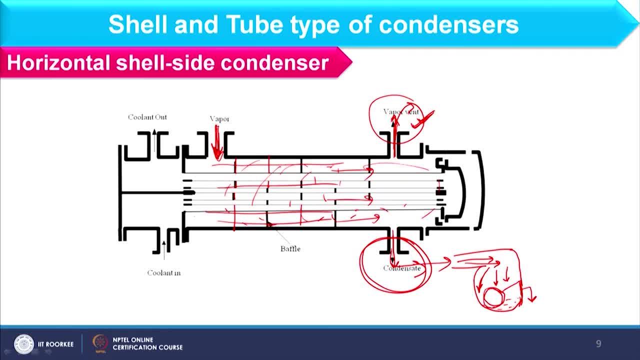 because this balloon is there. Okay, This is very light, So as this balloon moves up, it will open this channel, okay, And when it will be opened, condensate will keep on exiting from here. However, it will not allow any vapour to exit, because vapour is available in this region. 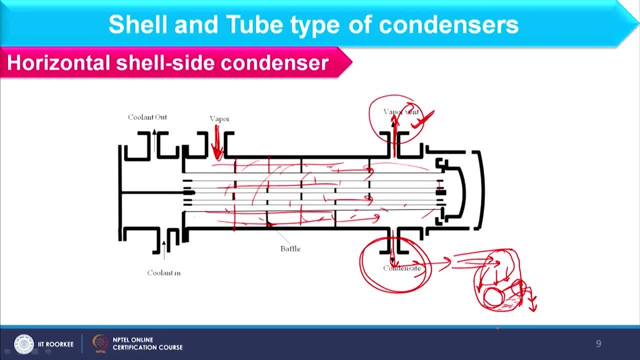 not in this region because of the density difference. So, in that way, steam trap works and we trap the steam or we trap the vapour, Okay Okay. So steam trap works and we trap the vapour and let the condensate to exit the system. 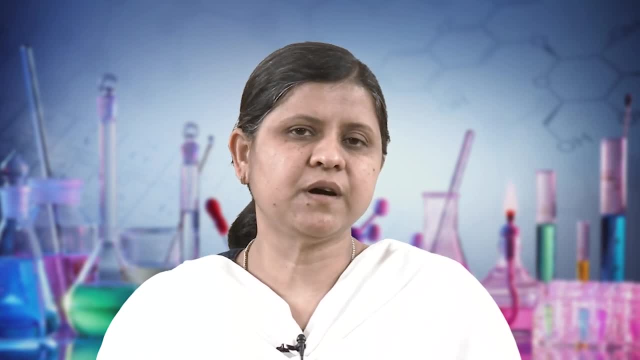 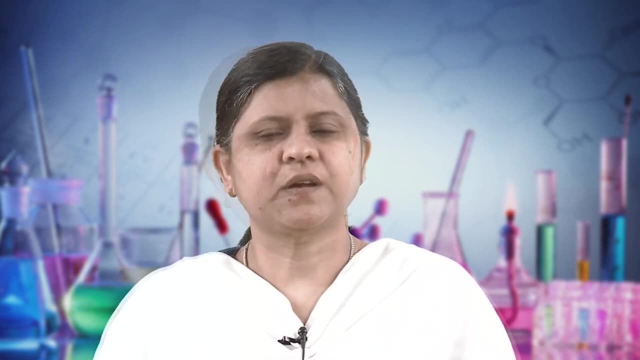 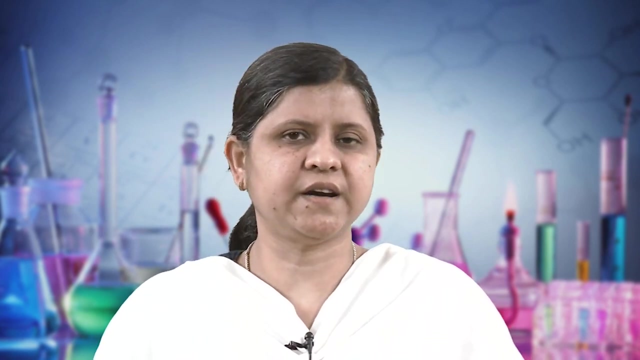 okay. So whenever I am using vapour and steam, I should use extra assembly in terms of vent nozzle and in terms of steam trap. So I hope you understand the function of vent and steam trap. and further we can consider horizontal shell side condenser, as it is shown in this schematic, where vapour is entering.